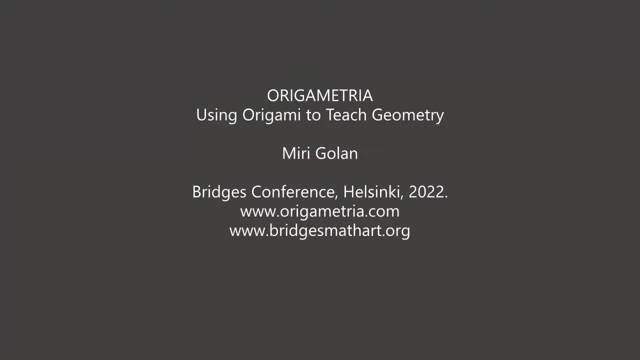 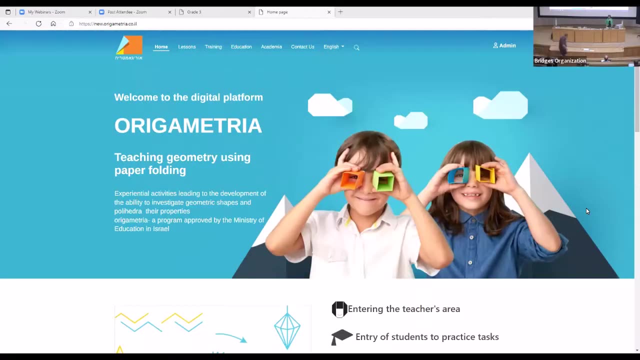 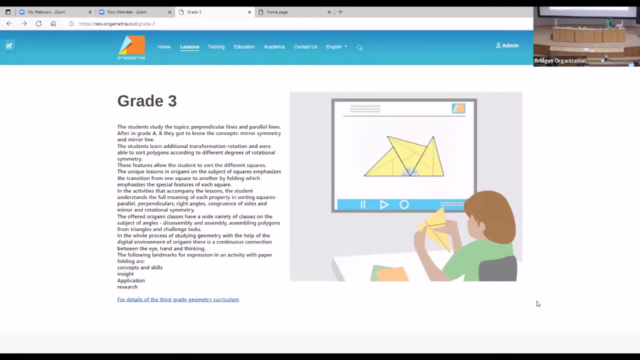 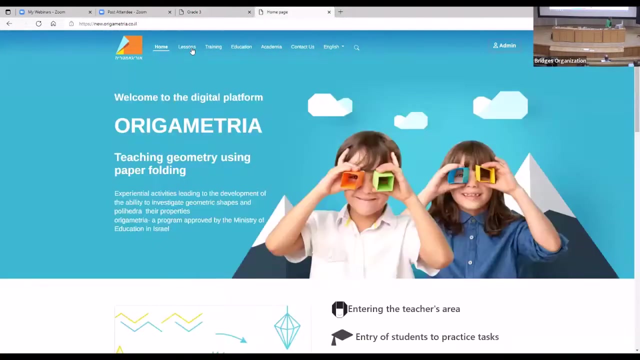 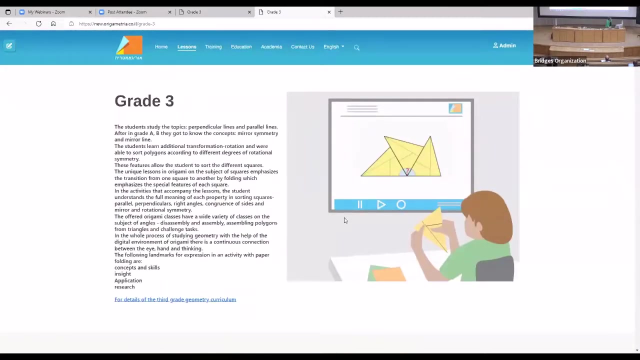 Thank you. I'm going to talk from the Orgometria e-learning site. and I'm going to talk from the Orgometria site. Okay, So what? you see that usually the teacher I go to grade three and the teacher in the class 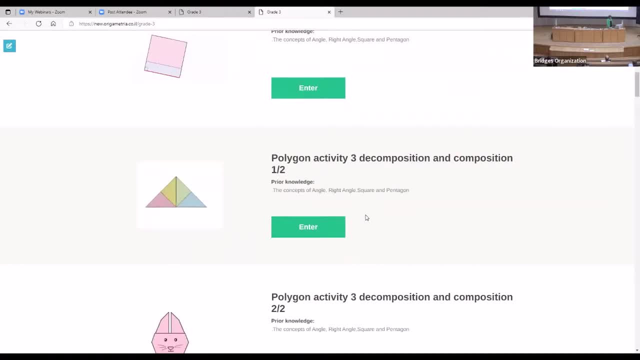 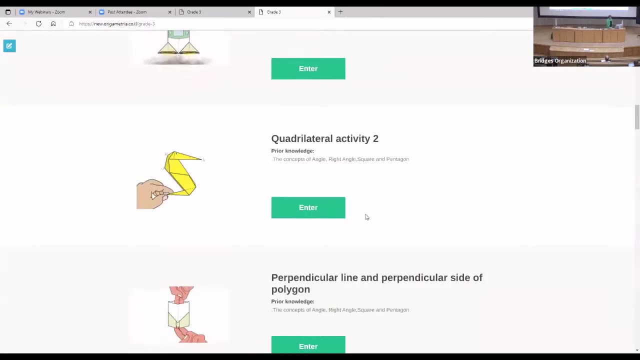 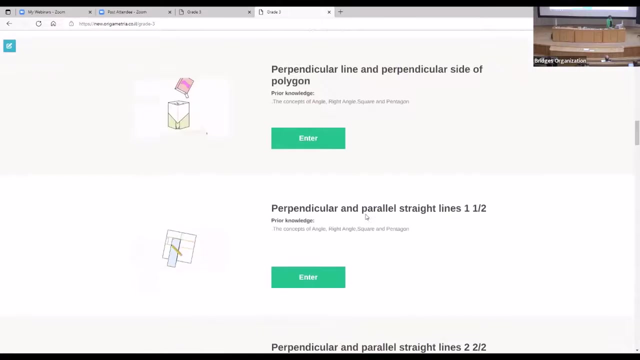 screen that, like here in the class and work with the student. If you see this rabbit, it's teach polygon. And the spaceship teach water lateral. and this bird and the books, each one of the model, teach some topic in geometry, like the books teach perpendicular. So today I'm going to show 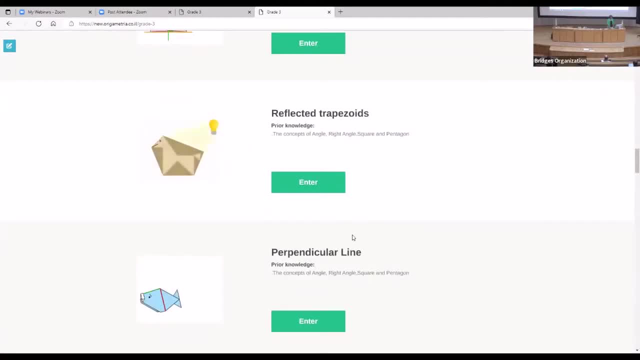 you some lessons we call reflected prophecy on. You go to paper, You see the result. I'm going to show you some lesson who call reflected prophecy. You go to paper, You see the result. but when the teacher come to such presentation, like Newton, I try to jump and won. 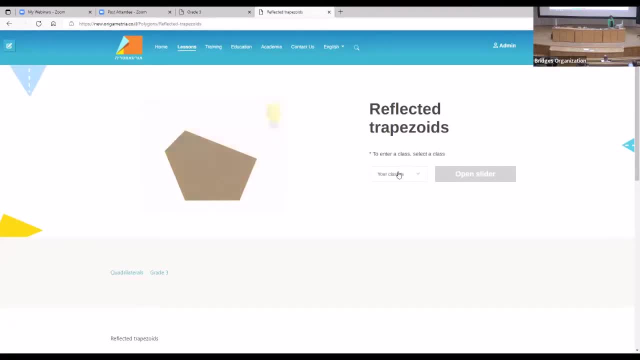 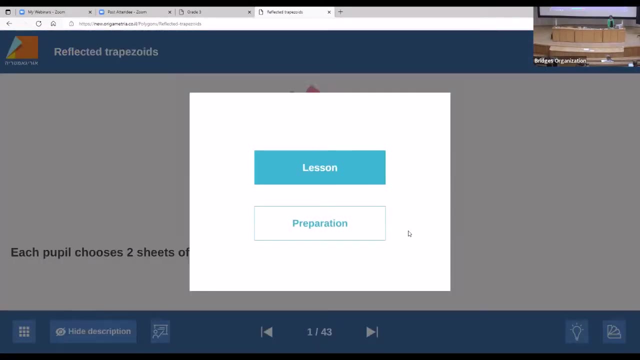 실제 your animation. that what the teachers live by slowly. I find you see that I can. PRO 카. come to the class. she opened the lesson. she choose the class, she prepare. it's called Helsinki Neri today and she opened the lesson now. usually she can prepare the lesson and write comment. 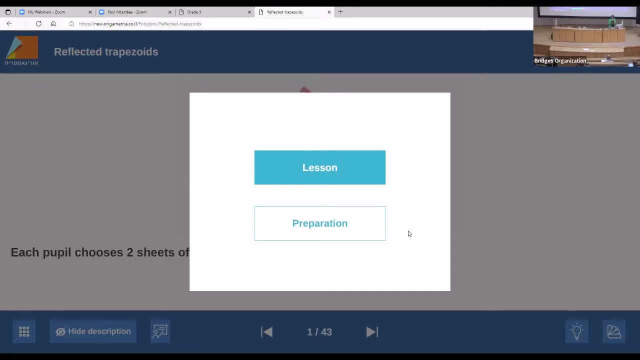 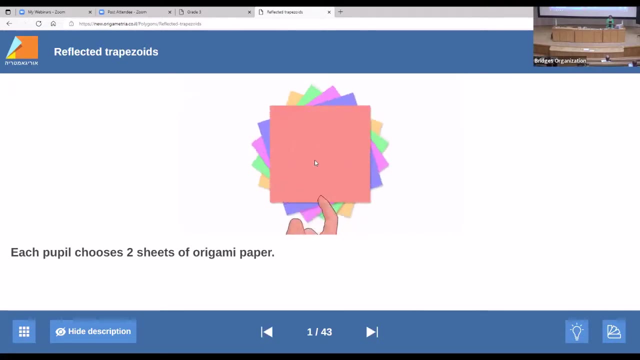 maybe she want to ask them some other question in the middle of a lesson. she can do it in the preparation. but because already prepared today, so I go straight to the lesson. and now she's in house, she hands to the kids the origami paper. so the children take the paper. 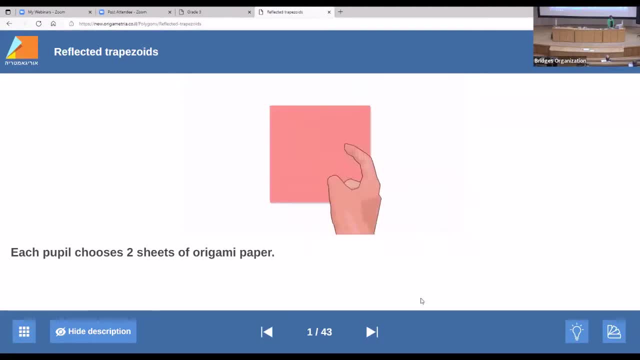 and she start to teach. you already got the paper. so one of the questions she asked them: what is the shape of this paper? so if I ask you, you say it's a square and I'll ask you: why is it square? you always have this question, question and answer. 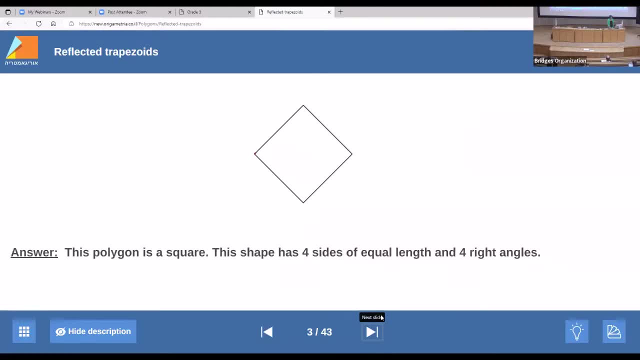 and folding instruction. so you say to me: okay, it's a square because all the side is equal. have a right angle, so it's a square. but how do you know all the side is equal? how do you know it's a right angle? we know from the PISA exam: many of the children fail because 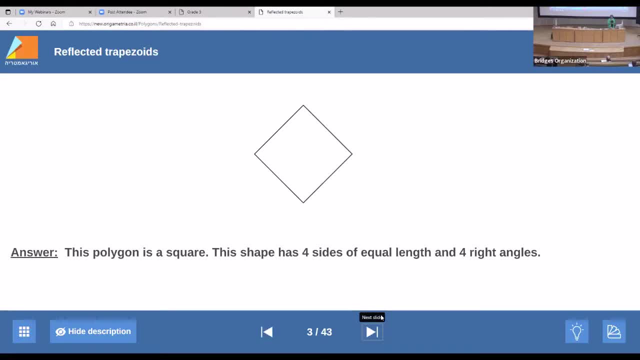 they say it's look like, yeah, and we, with the argument i deal with this, look like the children work with the hand and the virtual world in the same time. so how we can do it, how we can know this is equal side and right angle. so i ask you to take one of the paper you have. 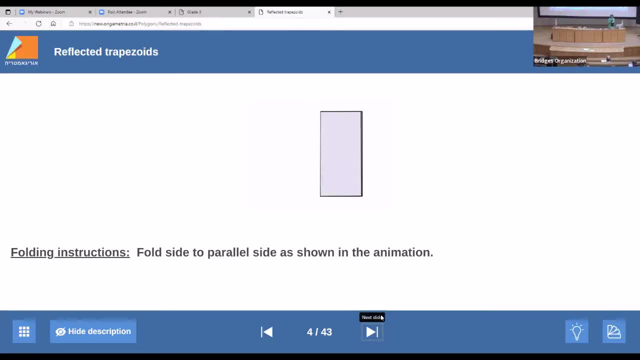 and fold one side to the parallel side. always it's better to fold on the table and not in the air, and i know you have small tables. so i suggest you to open your table and fold and you fold now long side to the parallel side and then, after you did that, 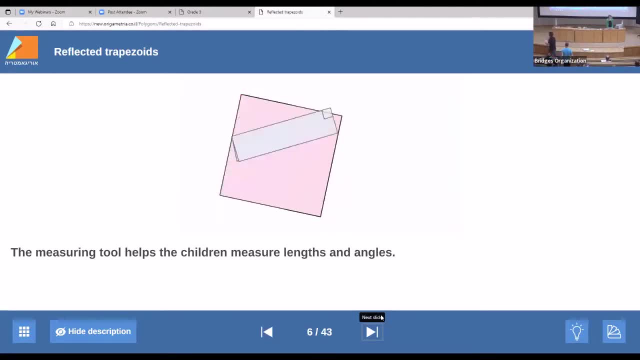 you put a sign of a right angle only on one corner. so if you see the- we call it- paper measuring tool, and every student have a in his bag. if he lost it, it's easy to make a new one. yeah, so now he can check that and say yes. 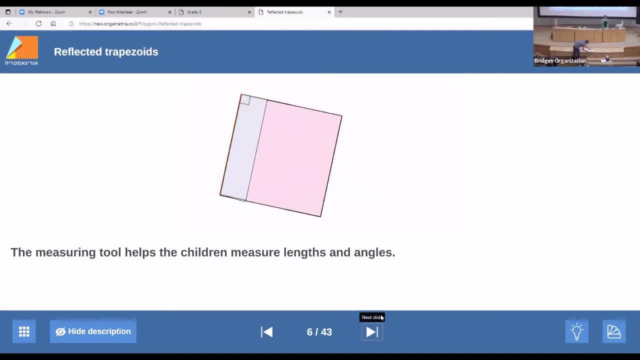 all side is equal and the angle is a right angle. okay, so after he checked that, then we know that. he know it. okay, everybody have a square, somebody don't have a square. okay, so the measuring tool. this is how we start now. the children doesn't know. we fold, what we fold. 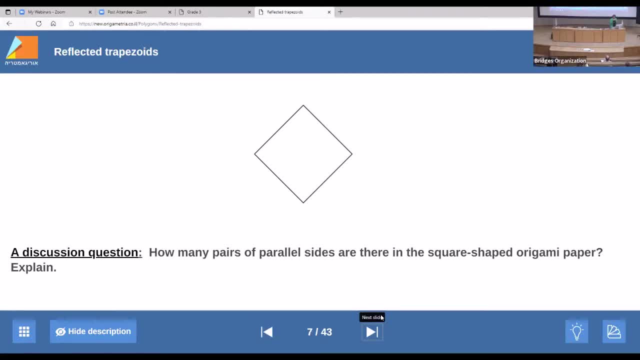 you see it in the beginning when i got into the lesson. why they don't see it when the teacher get into the lesson? the name of the lesson is reflective propesium. it doesn't say what's the model we fold if we want the children imagination to work- and we know the children have high 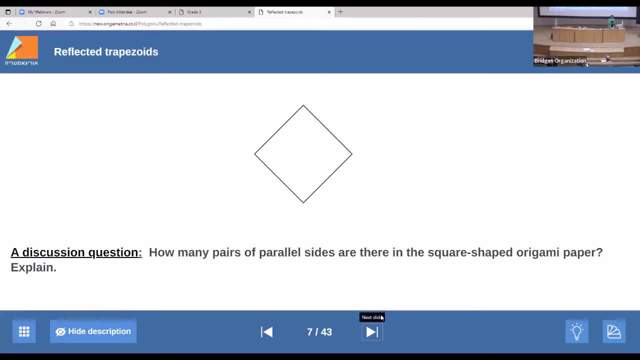 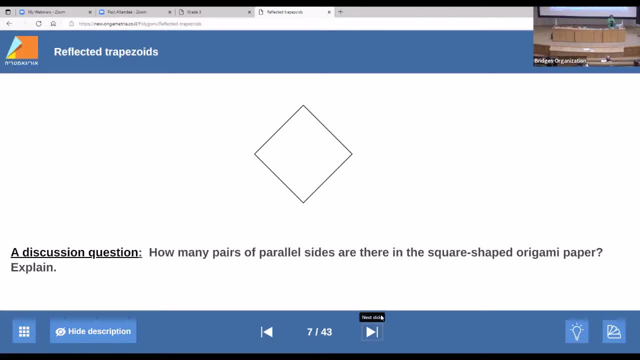 surprise. so each time the paper change, they get a different model. so now i ask you how many pairs of parallel side you have in your paper and how you checked it. so you tell me, yes, there is two parallel side, two pair of parallel side. this is one of them. 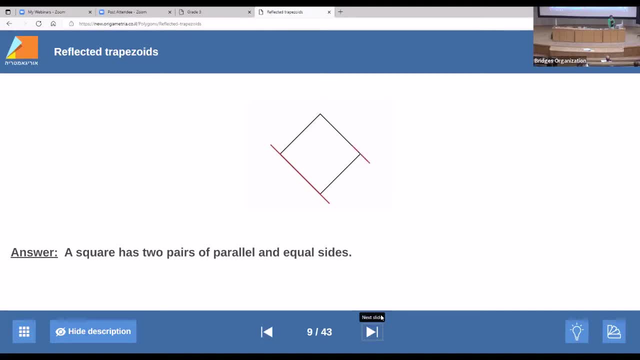 and this is another one of them. but how do you check they are parallel? why, if you show them in the square, all the children say it's parallel. show them a rhombus: say it's not around a parallel. yeah, it doesn't look like. so we teach them to take the measuring tool. 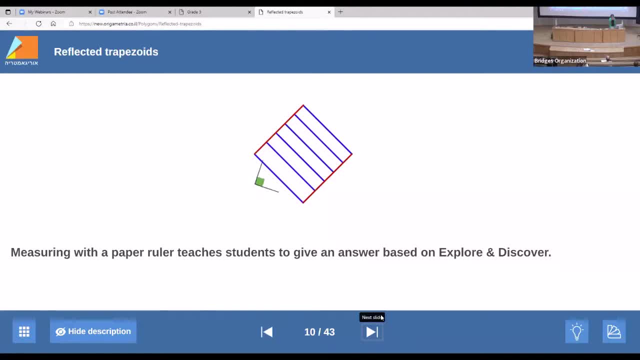 and make a particular line between the two side, and then you know the distance between the two parallel side is equal. so now we fall. take the other paper you have and fall one vertex to the opposite vertex. now i don't speak origami language because while we come to teach, you want to teach them with the mathematics language. 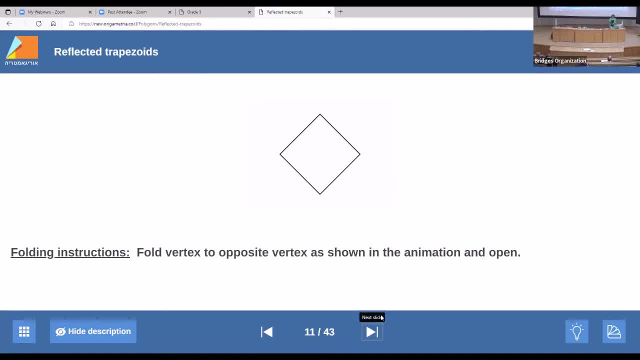 one of the beautiful comments i heard from teacher. they feel like they and the children have speaking the same language, because the children can read that, they read the question, they read instruction, the reader answer, and this is very important because many times we need to give them a good 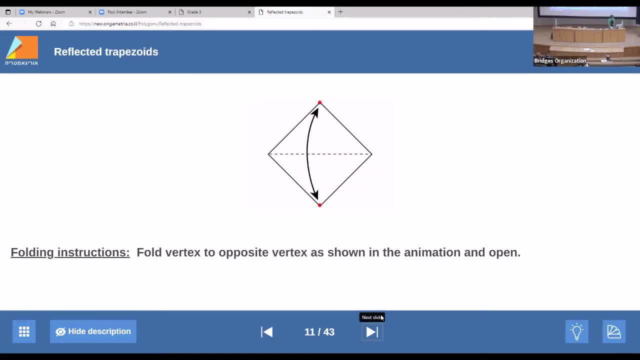 mathematics language, and if you know a good math teacher, you can give them a good math language and and they get used to that. so now we fold it and open it. and now what we do? we fold the side to the symmetric line. now, when you fold it, make sure. 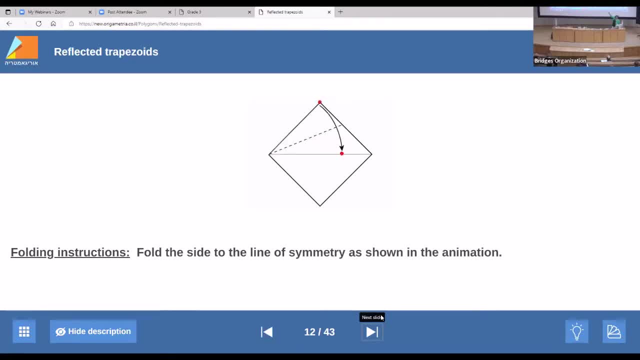 you fold in the same direction. you have here. okay now, if you see the light, the um, a balls, how we call it, if i put uh the mouse here. it's a comment. we give the teacher uh in the lesson if she want to remember something more, yeah, so now i tell the teacher. 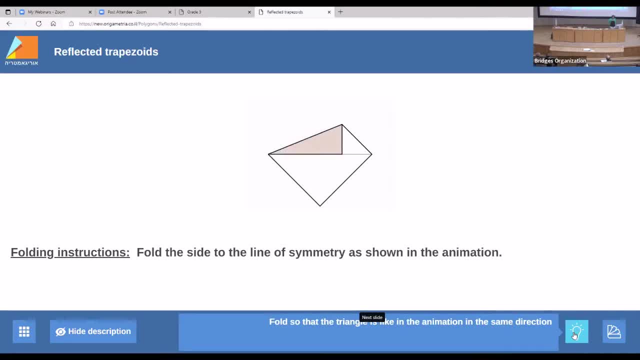 make sure the student fold it in the right direction. if i move the mouse, it's disappear. okay, if the teacher put her mark, she will see it in the other side. okay, if the teacher put her mark, she will see it in the other side. okay, if the teacher put her mark, she will see it in the other side. 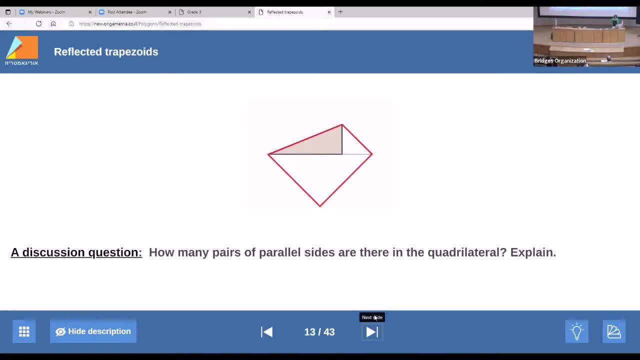 so after you fold it, i asked them how many pair of parallel side you see in the shape here. so the children check that, how you check that, how you check it in the rulers- yeah, paper rulers. so what we do? we put the paper rulers on the side of the paper and we put the paper on the side of the paper and we put the paper on the side of the paper. 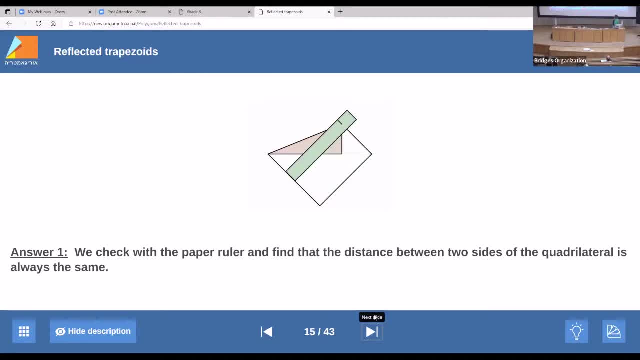 on the side of the paper and we put the paper on the side of the paper and we put the paper on the side of the paper, on the side of the paper and we put the paper on the side of the paper on the shape we did and we mark it. 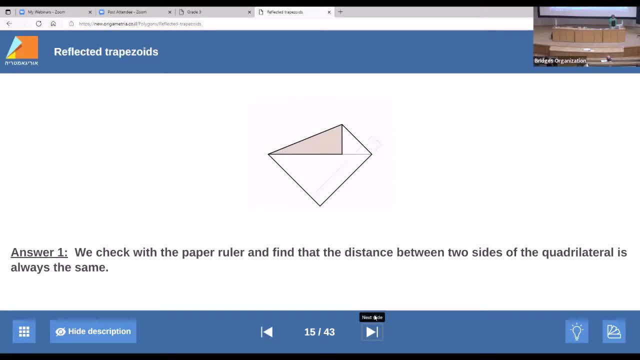 on the shape we did and we mark it. on the shape we did and we mark it. and we see the two sides are parallel to each and we see the two sides are parallel to each and we see the two sides are parallel to each other other other. if you check it, we know it. 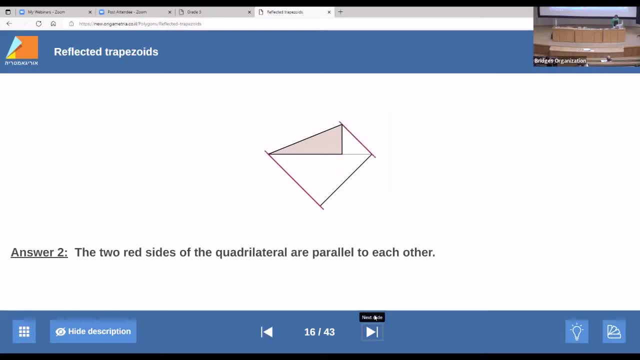 so now we check the other side. no, this, sorry, this is the parallel side. no, this sorry, this is the parallel side. no, this sorry, this is the parallel side. this is how we mark it, and now we check. this is how we mark it, and now we check. 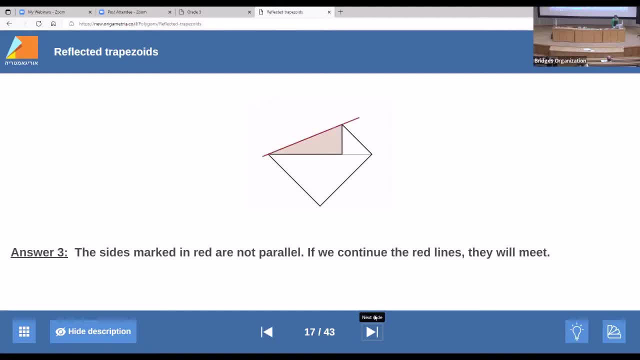 this is how we mark it. and now we check the other side, the other side, the other side, okay, and now we see that if we continue, the two line can meet. so this is not a parallel. so just now we say: what is trapezium? part of the um? i remember i teach in los angeles and ask the children to make a square and ask: 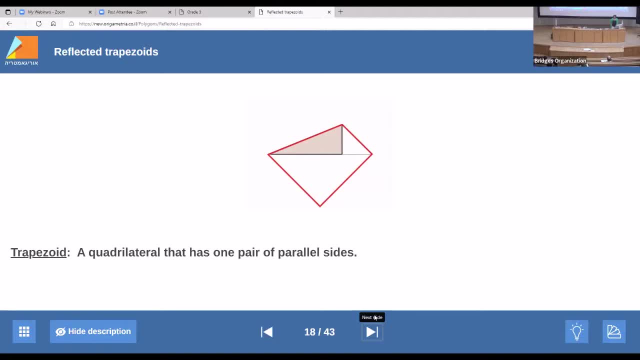 them what's that? he said. they say it's a square and ask the white square. and they said: because the square. they try to remember what the teacher told them. if you teach by repeating by memories, you teach nothing. but if the student investigated and checked it, they never forget it. 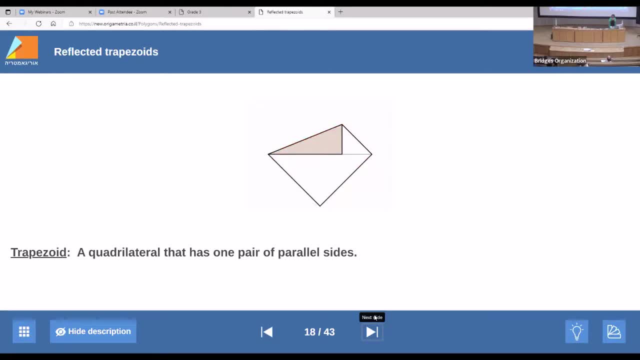 so here we check the parallel: how many pair? and we saw in the square they have two. and we saw in the trapezium we have one. so this is how i build the knowledge you. so now what you need you to do: to fold the vertex. 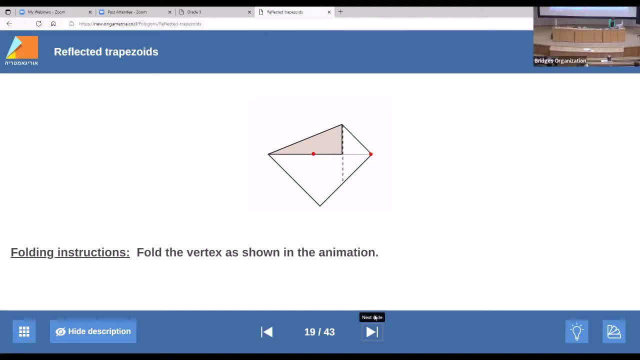 is it show in animation. now i want to show you something more about this animation. he worked very hard on it. the animation repeat again and again, and again and again. so if the teacher want to go between the children and see that everybody is okay, so she can the animation continue to show it again and again so the children know how to do it. 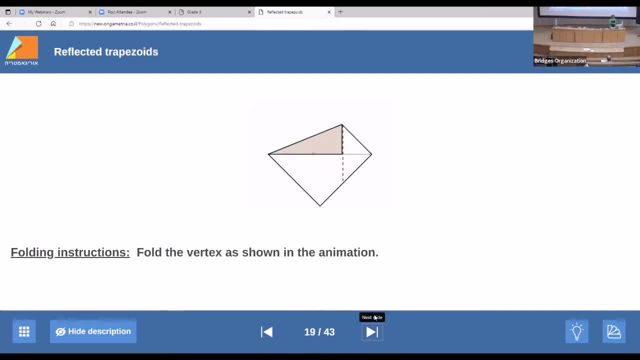 the model is created by paul jackson and he do all the work with the animator. okay, so now how many pairs of parallel side we have in this shape? so how we check that? so again, we look at the two sides and we see that if we continue they can meet. 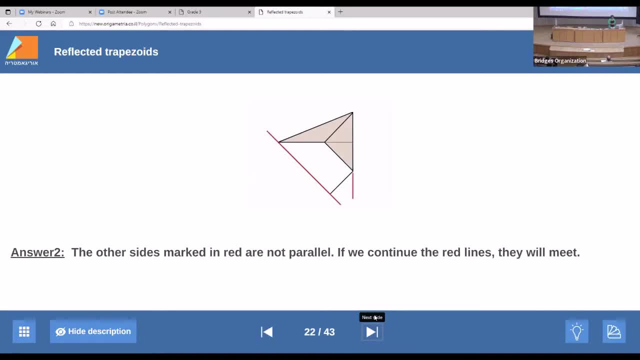 and if i see the other side, they also can meet. now it's look a bit like trapezium. yeah, if you ask children, they say trapezium, but it's not because doesn't have any. so when the children check that they never do mistake. 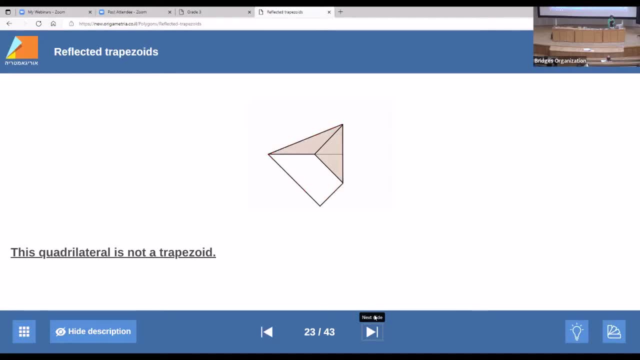 so it's quadrilateral but it's not trapezium. so here you can see that it's not. so it is not, finally, even, and of course when the children check all the other side, that they don't know to repeat, and if you imagine that the boy becomes larger and the other is larger than him, 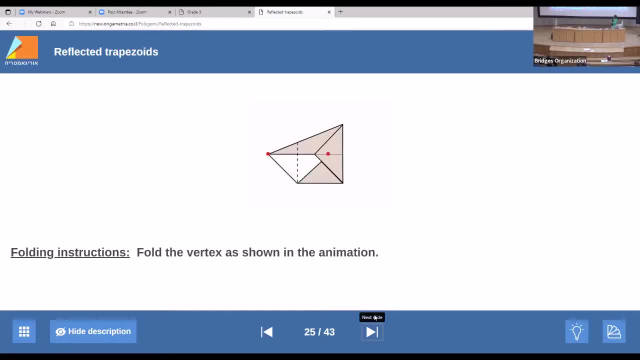 you would know what i mean and as you can see that and in the action. Now, if I ask you, is it important to accurate in origami? Probably all of you will say, yes, it's very important. And I say to you, no, why not? 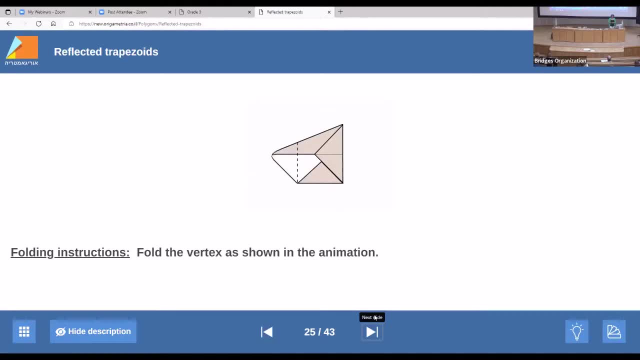 People who get annoyed if they are not folding accurate: it's people who are very, very accurate. They want everything to be precise. People who don't accurate: they just fold and say it's okay, They don't see it. If I come and make a comment to them, they get frustration. 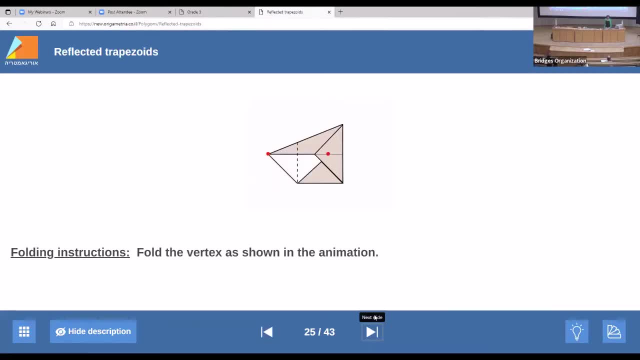 I never saw anybody who learned from frustration. That's why I never check. And the student asked me: is it accurate? And I say: I don't know. what do you think? Is it accurate for you? Is it okay? No, it's not. 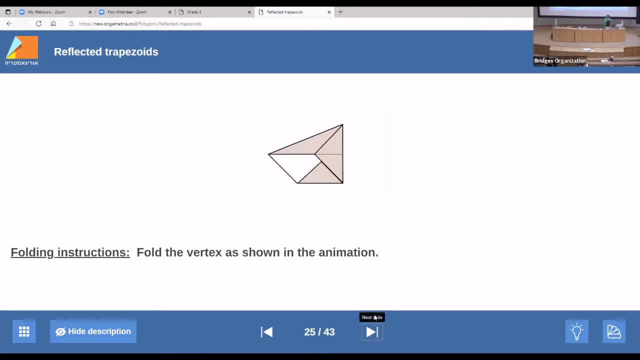 Okay, So fix it. It's not me, It's you, It's your work. Another thing we do: there is a lot of method that I don't have time to tell you about it, because origami come with an important method. 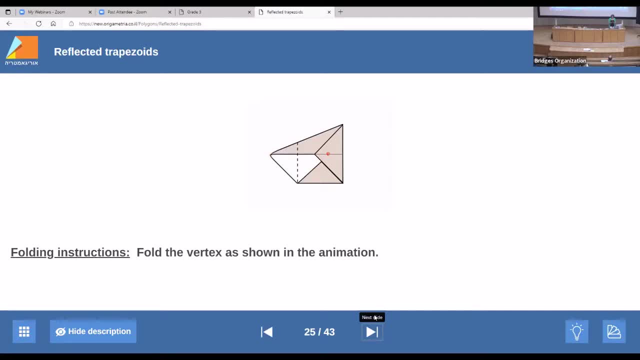 So it can make the student feel good about their work. We never touch the children work. I don't know. if somebody come and teach you origami and they couldn't make it, then he took your paper and make it. It's terrible. 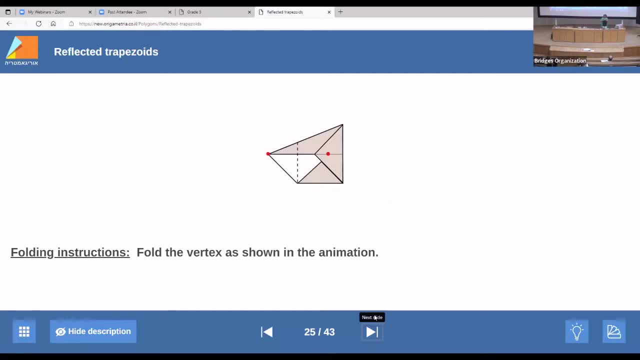 When I trained teacher, math teacher, And I really all the time tell them you're not allowed to teach to touch the student work. So they tell me they put the hand behind the back and they don't breathe because the reflex is to touch. 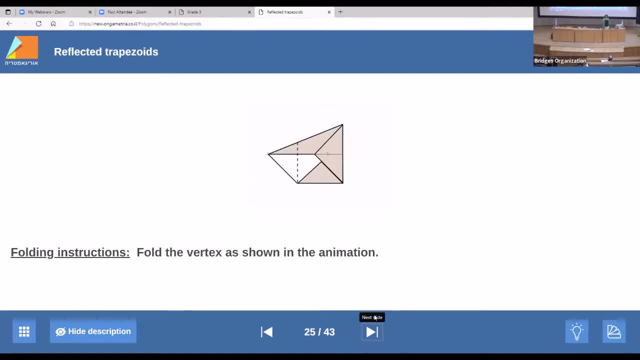 And math teacher tell me I stopped to take the pencil and make a right on the notebook of the student- that I never understand why they do it. Yeah, They usually don't have a understanding, But after the experience They find it's better to teach without. 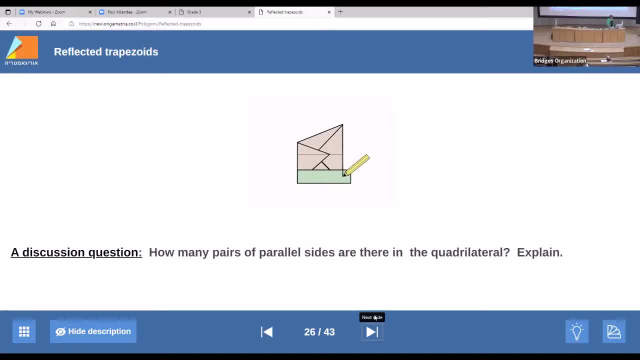 So after you got it, we check again: is this how many parallel side we have? So we check with the measuring tool And we see that this side is parallel, two side parallel. So this is how we mark it. And then we look at the other two side and we see they are not. 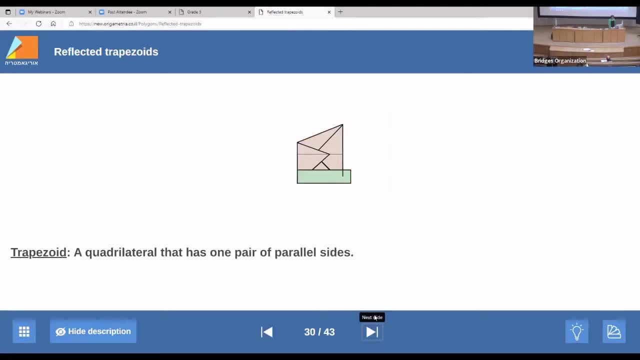 So what do you think, Is this trapezium? Now, the children know what is trapezium. they never forget. Okay, So now we open all the fold we make And this is very. this is one of my favorite part, because if you look at that, you find 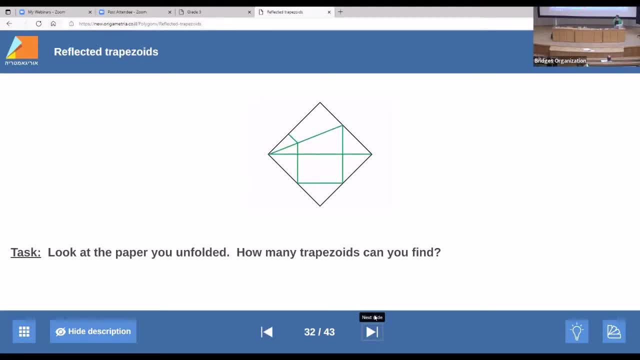 many trapezium. Some of them look like, some of them not look like, and when the child open it, try to find it, find to discover. it's a lot of learning. learning have to be by research, discovering, Yeah. 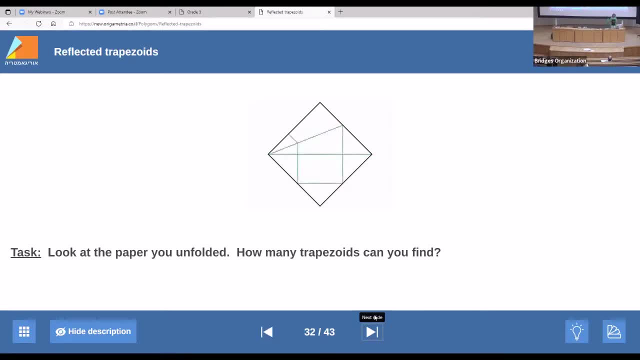 Not, but what I tell you, It's by what you find, what you discover. this is a learning. So now they can look at that and try to find out. And I never showed them Where's the trapezium here? 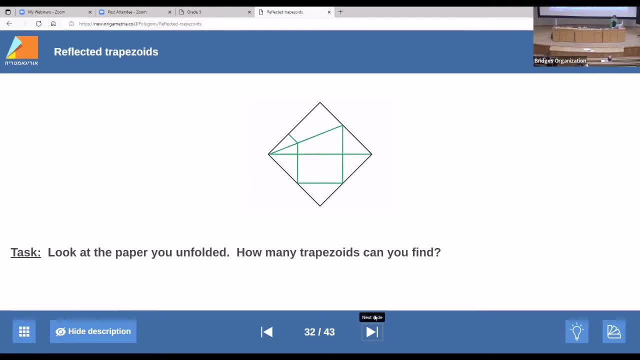 Yeah, because I want them to go home and think it's more trapeze. I want them to work Like this. student asked me a question. I never gave them an answer. I always say it's very interesting. what do you think? 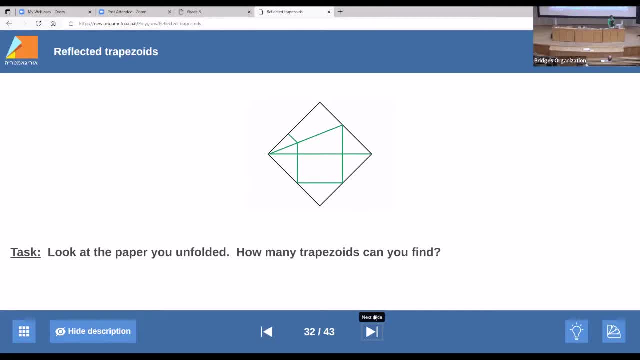 I like them to think, to think, to think. this is the most important. So now we continue to fold, but when we finish the fold, you can open and look at it again. So, look, make sure that you fold the vertex. 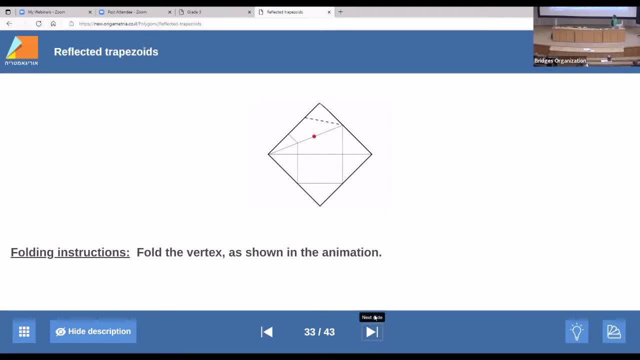 and it's showing the animation. Okay, That's why it was important in the beginning to fold in the same direction. Now, all the modeling, the augmented, are very simple, very beautiful. we'll create them And it's easy for the student to make them. 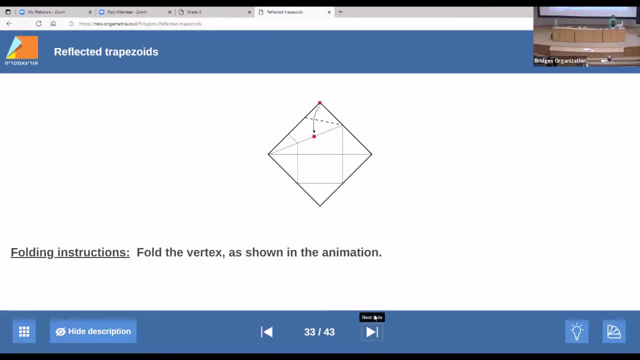 and for the teacher to teach them The lesson, the geometry in the lesson. it's built with Dr Johnny Oberman, who writes, is one of the writers, one of the writers of the curriculum in maths in Israel. He have 60 years of experience. 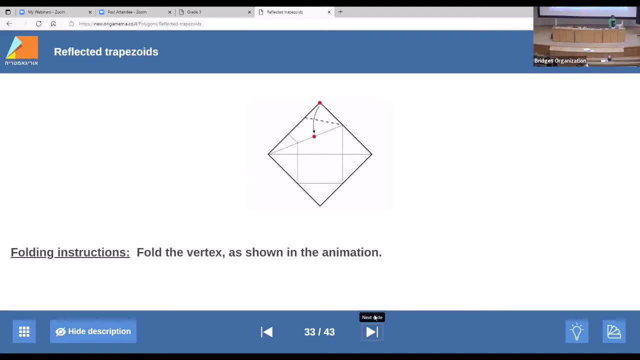 and we put all of it in origami and I'm very proud of that. Okay, So now we fold. after you fold the small triangle, you fold all the triangle as it show. Okay, Now, if children fold it and they need help, 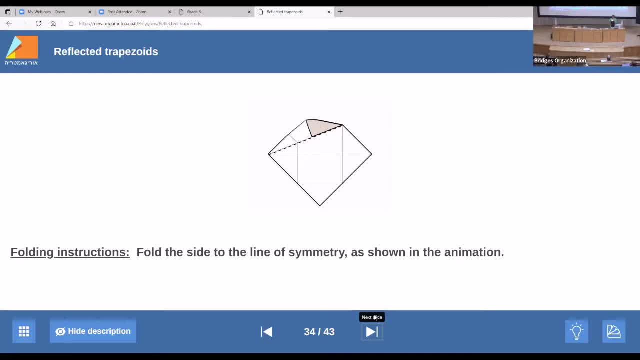 I don't touch a children paper, but I come to him and I hold my paper in the same direction as his paper and show him with my Very important Okay, So now I fold the side, You have a triangle and you fold the short side. 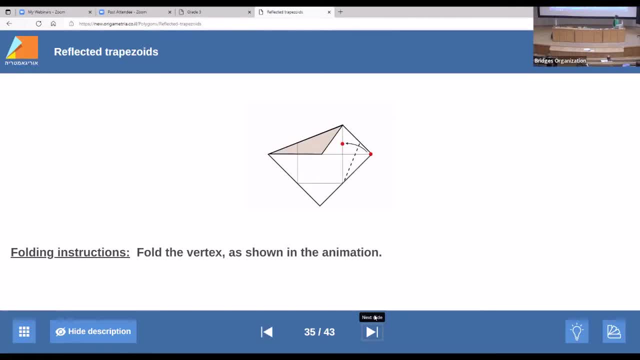 to the long side. So you see, all the lesson here is mathematics language. It's very important. And now we just close the small triangle. Do you know you are the first people who see the origamatery are new. Okay, So we have a lot of learning side. 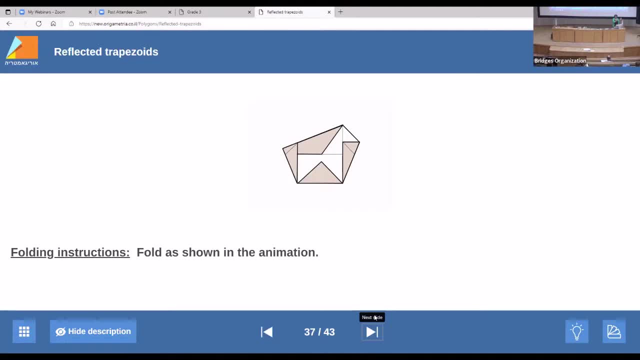 because we have another digital side and we soon another two weeks. we launched a new one. This is the new one, So the first people in the world who see that, And today I came here the first time I see it on the big screen. I got really excited. 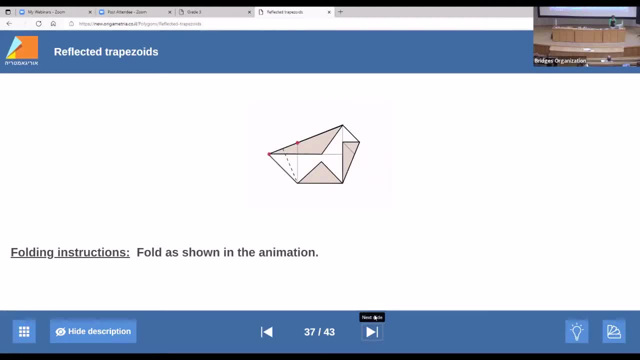 I put hours and hours, all my life I put in it. So now we fold the side to the line as Joe, And now we want to make to the horse small tail. So we tell the small vertex and we fold it. Hope everybody have a horse. So you know, children very creative And what we put. 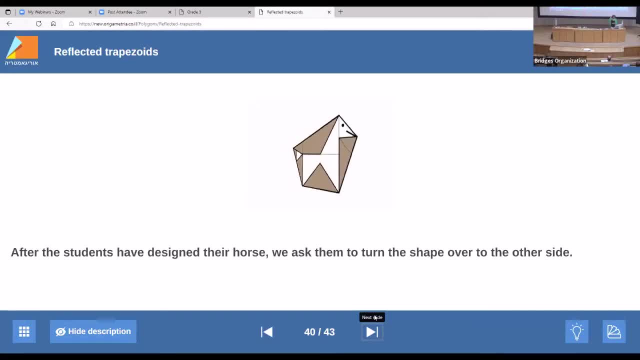 here only small dot in the line And I asked the student: can you design the horse, Can you put your own design on it? And you can't believe what children can do. You know I did that. I'm not very good, But the children put a lot of beautiful design, So the most 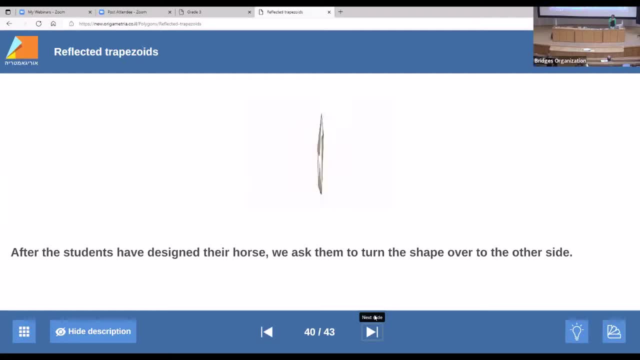 important. I said to every adult: never draw on your work next to a children, Never. If they ask me, I said to them I don't know how, And I put the crayon next to them and go And they draw. amazingly, I have a big collection of children drawing. It's incredible beautiful. 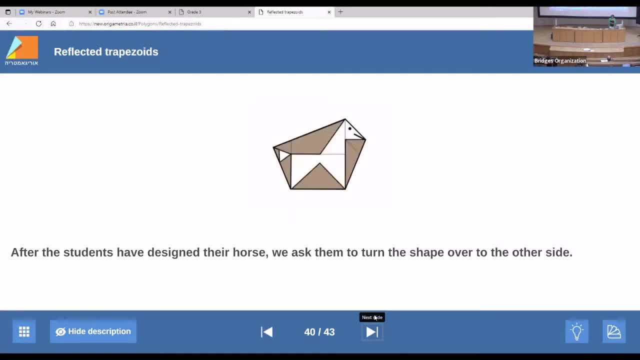 The way they draw, how they draw. it's just incredible. That's why, in this part, I want them to draw their own. So all the lesson, the paper changed the shape and they say, ah, it's a butterfly, Ah, it's a frog. It's all the time They start to think what it is. 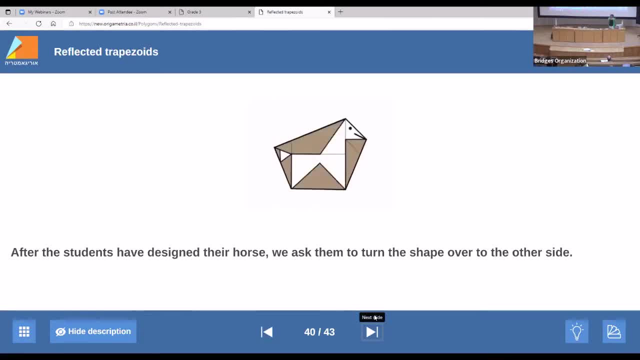 what it is. what it is Because origami- you tell them each step what to do. yeah, So how you be creative with origami? by not tell them what we're making. So they're all the time thinking what I'm making, what I'm making. Then they go this horse And now everybody can. 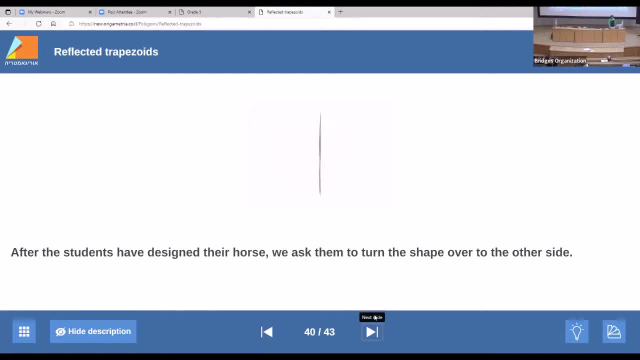 put his own touch to this horse. So if wait a minute, If you put a light, you can see the horse from the back. So if you look at the light, you see the horse. Take a picture of you. Where's Paul Come from here? You see the horse. 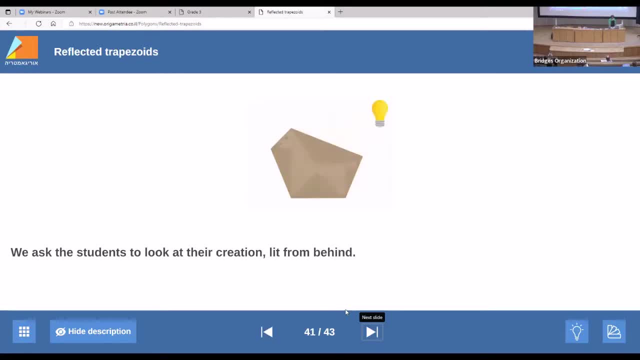 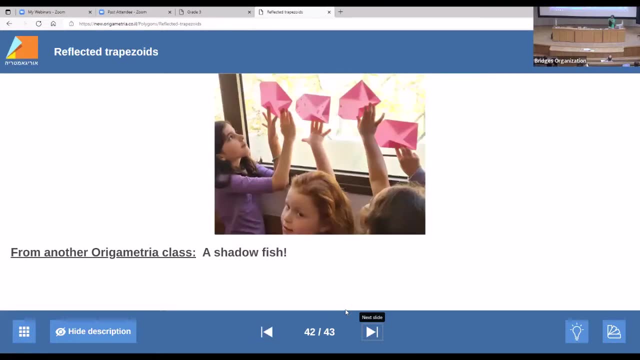 So if you design it, it will be more beautiful. So we did a similar model. It's a fish, And look what the children did: They run to the window and start to look at it from the window. This is some of the teachers send me. They design the fish and look at it from the window. 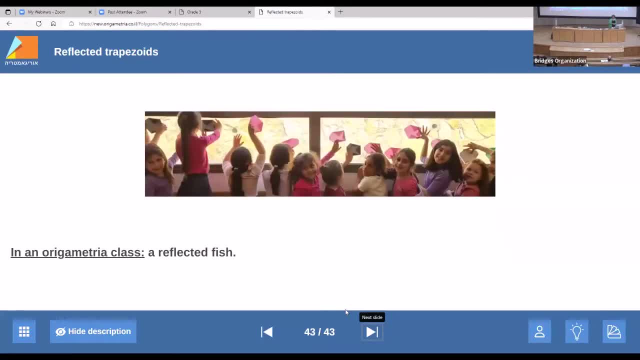 And this was just. they run to the window and it's beautiful to see it, Yeah. So my question: did I teach them what is trapezium? Did they ever forget it? And what did they learn? They learned to check, Yeah, And sometimes the lesson finished and the children still investigate and learning. 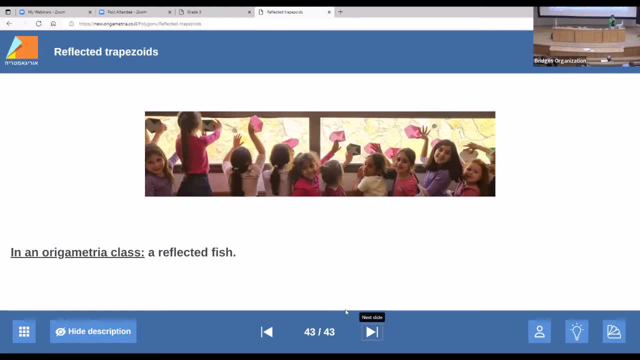 and try to find it out. The argument is: from kindergarten to middle school. kindergarten It's a bit different but it's beautiful, And one of the kindergarten teachers say to me that one of the kids who's not participate and not very active, uh, they moved to a new house. 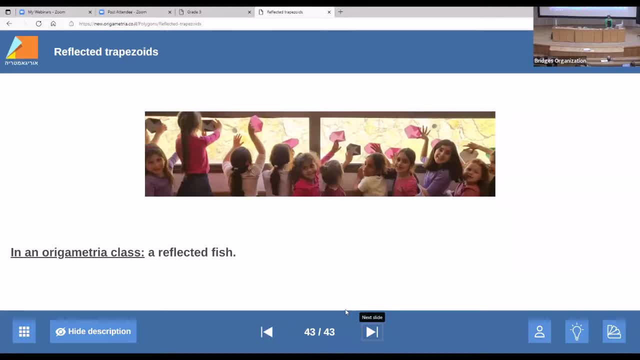 So they went to the new house- house empty and the kids run to the living room and look and say, look, mommy, it's a lot of square here, Look the the the right angle and start to run around the house and just look at the tile. 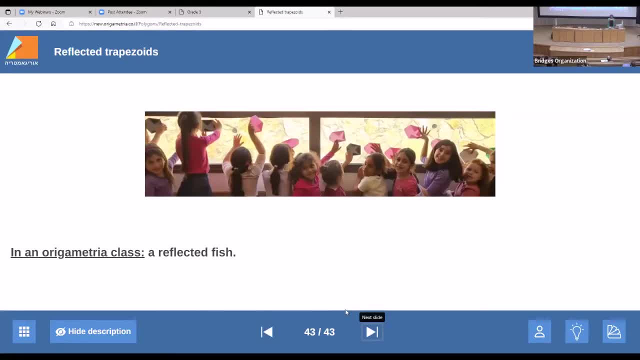 It doesn't look at the room anything, because what we did? we play with them, with geometry. So the geometry is interesting and it is- it's the most excitement, I think, topics. So after I show you what is origami lesson, I can talk to you about origami. 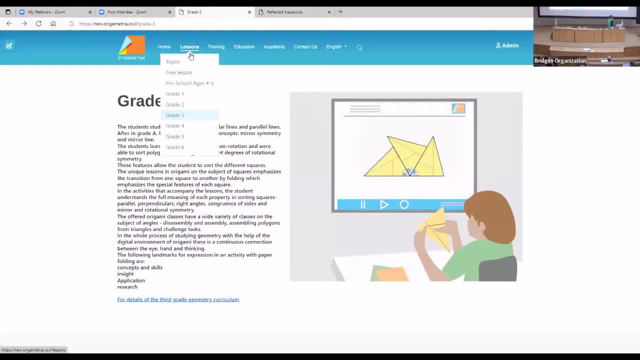 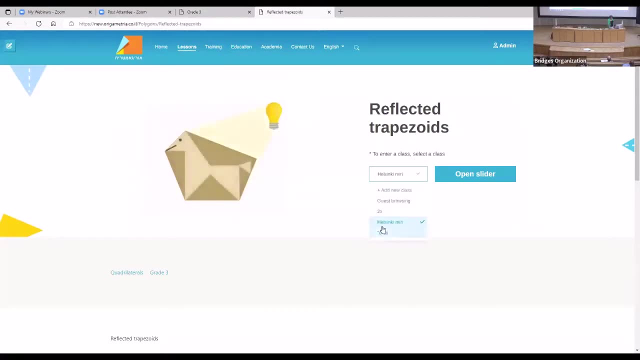 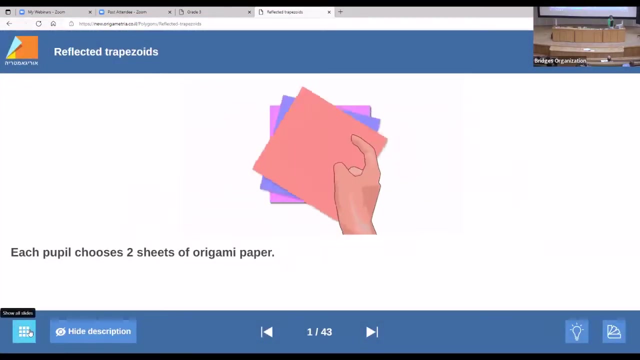 So I go back this one. I go from here, So I close the lesson. By the way, I need to show you something. Um, if the teacher wants to see all the step, she can press here and she can see and go to a certain step. she won't. 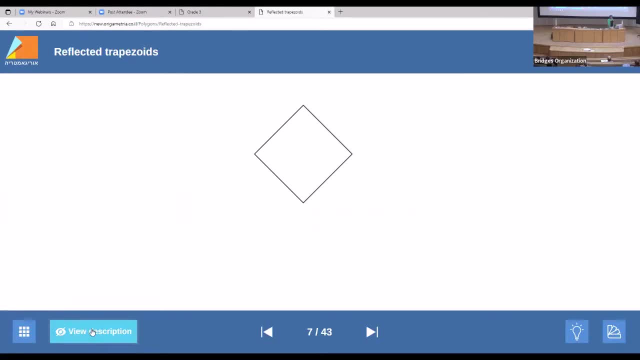 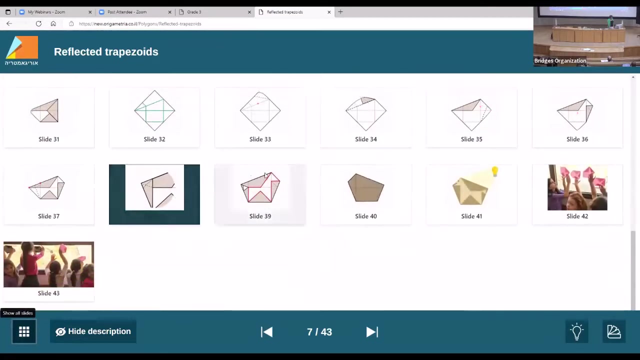 If she wants to hide the text, um, she, so the text will go. if she doesn't like the blue and she want orange, she can change the color. yeah, when she finished to teach the lesson, let me show you here. go to the end, almost to the end. 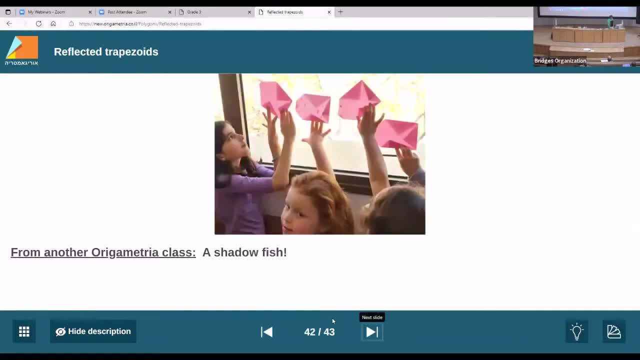 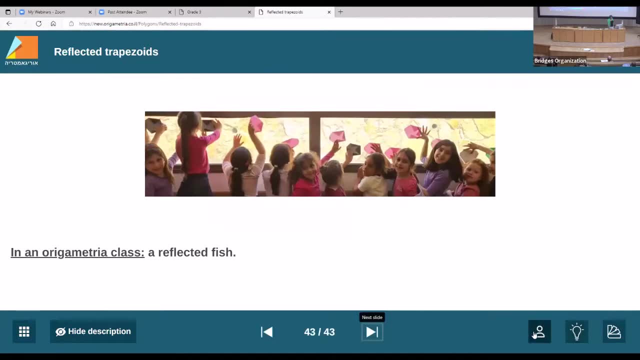 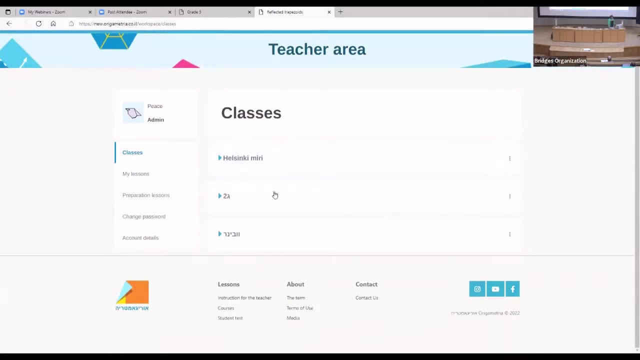 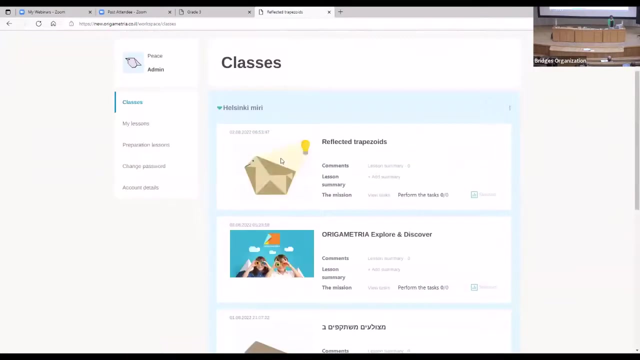 usually in the end: oh yeah, here it is. you see the teacher drawing so she can go to her area and all the school she, all the classes she teach, it's here. if she press on it she find all the lessons she check. also she can send some quiz to the student after. 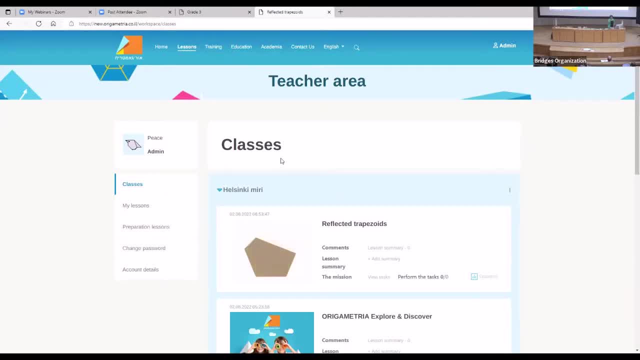 she teach. so they need to answer that and then by the answer she know if they understand the topic. but in the end of the quiz they have the step of the folding we did because the children doesn't want to go home and just answer question. they want to make the holes we make today. 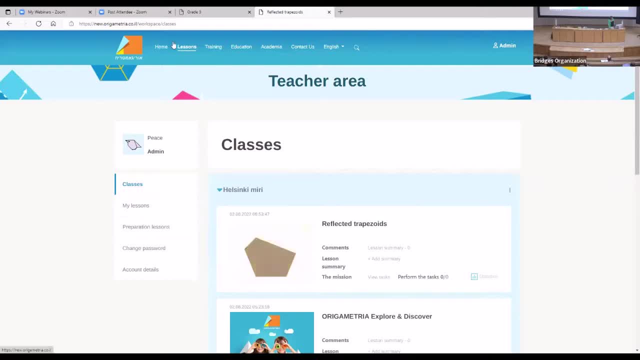 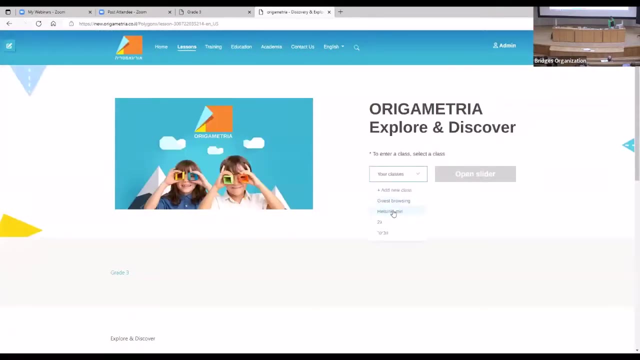 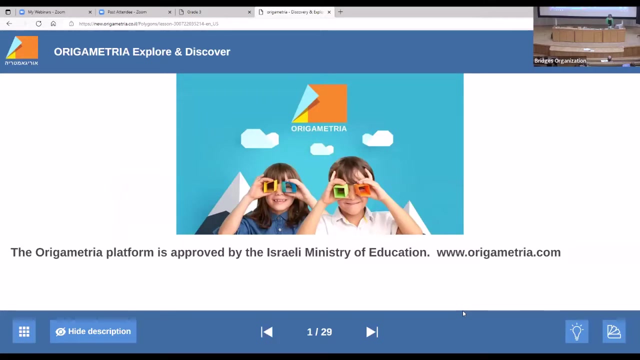 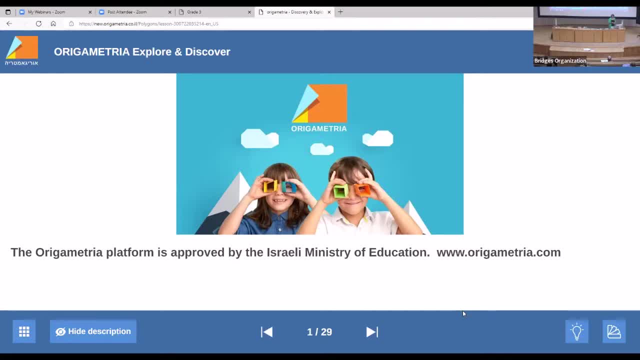 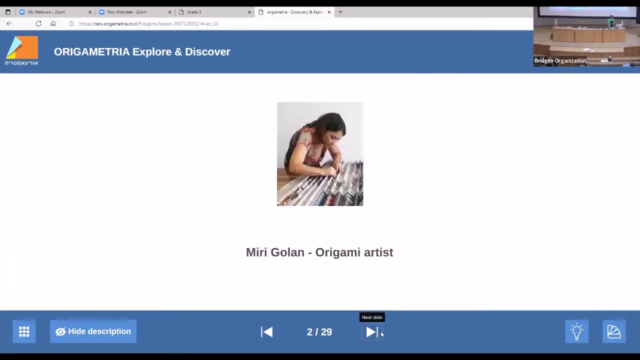 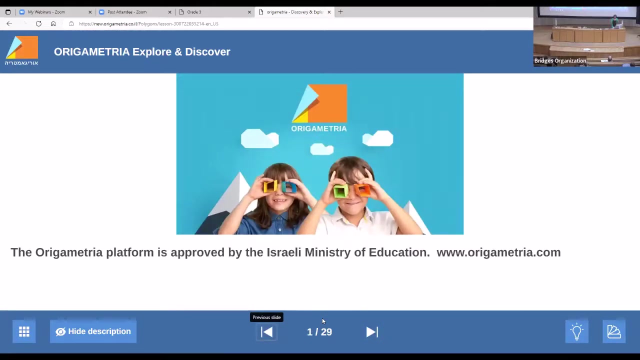 curriculum and we have about 160 000 students who study every year. we have more than 600 school and it's the four years the school renew the membership in the site. we usually sell them a membership for for one year. um, if you go on the online, you don't see this one, you see the old oligometric site and after two, 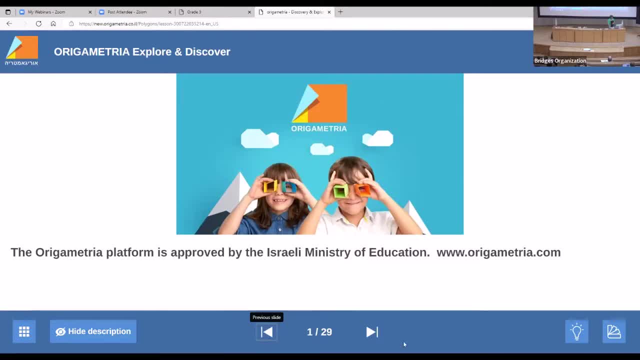 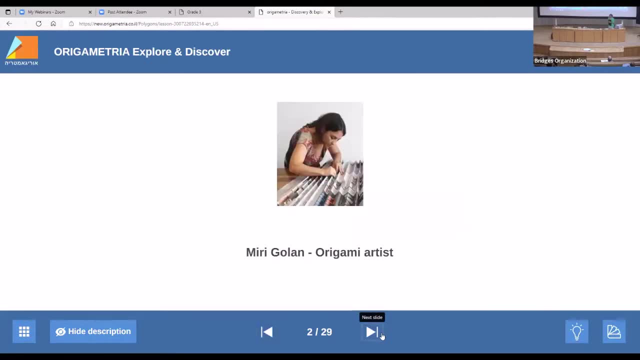 to three weeks you get a new one, but the old one is beautiful too, i have to say. um, so who i am? i born in jerusalem, in israel, grew up in jerusalem. when i do art, i'm an origami artist. when i do art: it's come from the people i know. i i grew up in this city. i grew up in this city. i grew up in. i grew up in jerusalem. so when i do art, i'm an origami artist. when i do art, it's come from events. 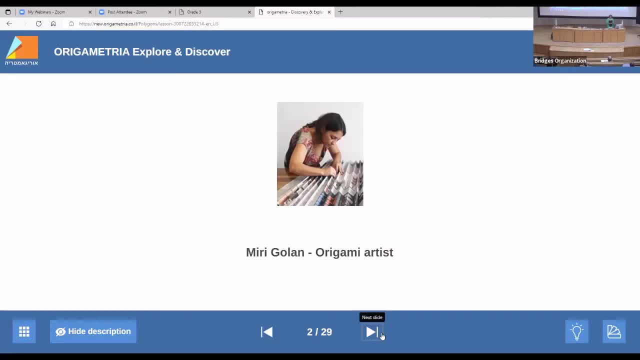 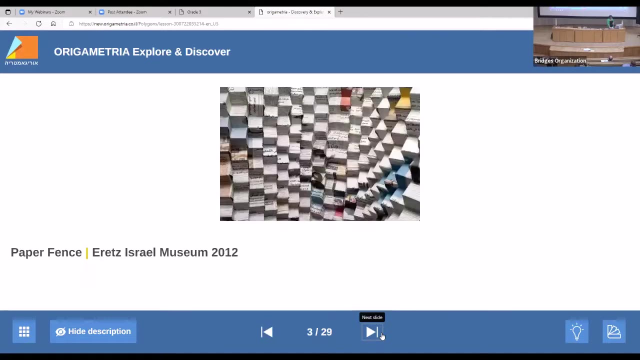 my region, for my, the way I live, the way I grew up in Jerusalem. since established the origami center, we work with Israel in Palestinian, Israeli, Arab. we work with all kind of population in Israel. this is a artwork that I did on a newspaper: one side Arabic, one side Hebrew. 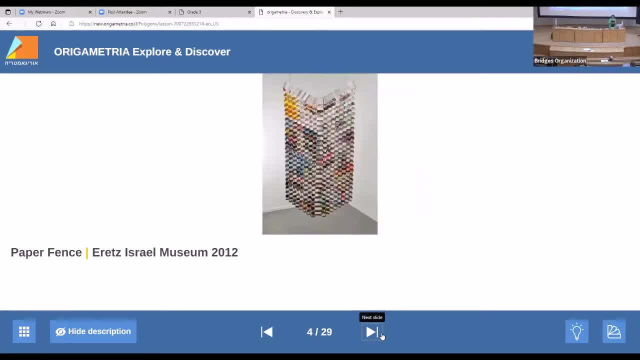 and it was in a museum and I called it paper fence and sometime I used to stand there and people didn't know I make the work and I like to hear what people talk. and some people say it's so nice when the Arab and the Jewish together the language and some people say, oh, it's really. 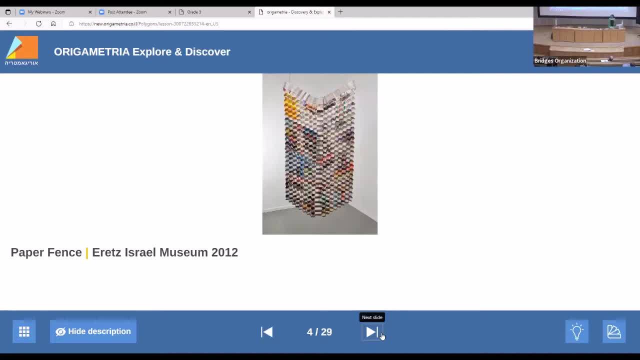 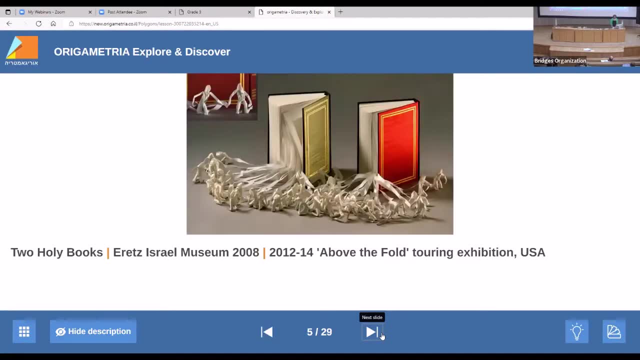 once against each other. so it's depend what their opinion. this is what they think about my work. I like it. this is two holy book and from the holy book I cut a paper. it's a handmade, not text on it because the word is word of God. so I don't put text and I cut the paper, the paper and make all the men from there. 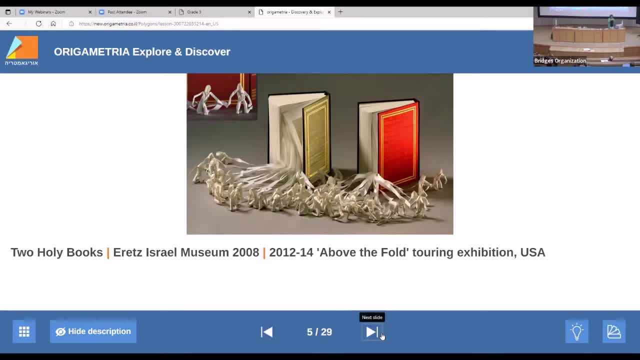 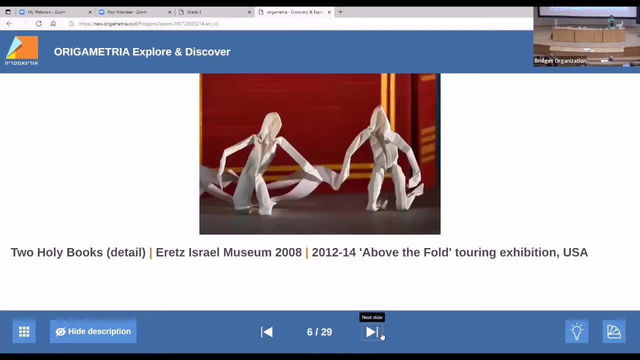 but the man is still connecting to the book, but you cannot know which men belong to which book. this is the two men who's coming from the whole book. it's a exhibit in the museum in Israel and been in, I think, 14 museum around America for five years and now it's in the 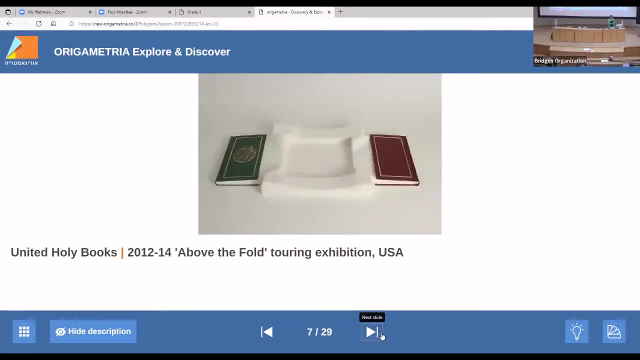 museum in South America. this is another two holy book. that is actually one sheep I like to fold from a bible paper. I like the touch and it's very special and it's cut the same sheet. move to one and another book to get the connection between the two books to different holy book. 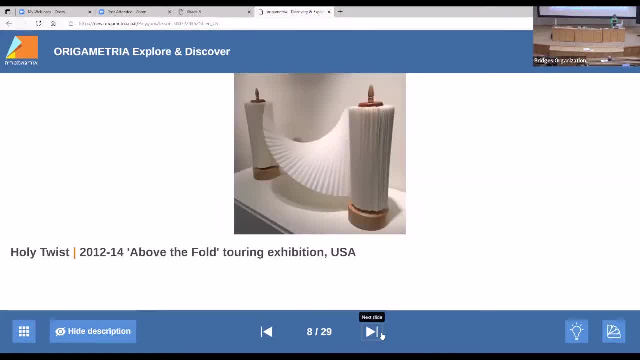 this is my favorite work. this is the door. the Jewish door- usually it's in the synagogue- is closing the carbon, but in the middle is not waist strike. now the two walls made from a bible paper. but I bind, handmade binding while I fold. it is to be a circle. the middle is the same material. they make the bible from: a leather of a cow. 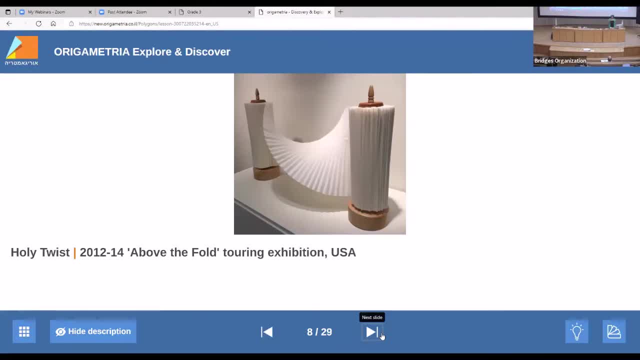 but i twist it and this is my way of saying that you twist the religion, or. but many times we've been to port in museum and many times i've been invited twice to open exhibition with that. it was part of origami exhibition. paul exhibited that too and i like 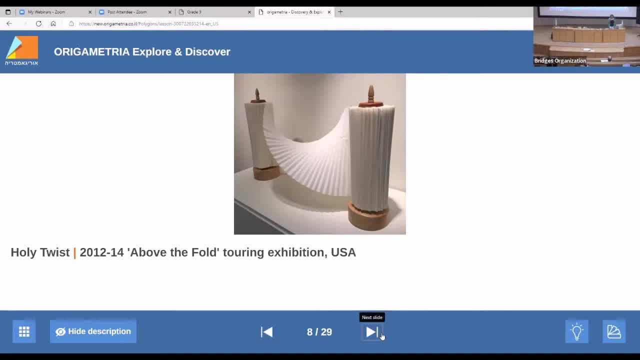 to see the comment of the people, how they think. i like them to think about it because this topic is burned inside me and i grew up in jerusalem. so in 92 i established origami center. people didn't know what is origami in israel. 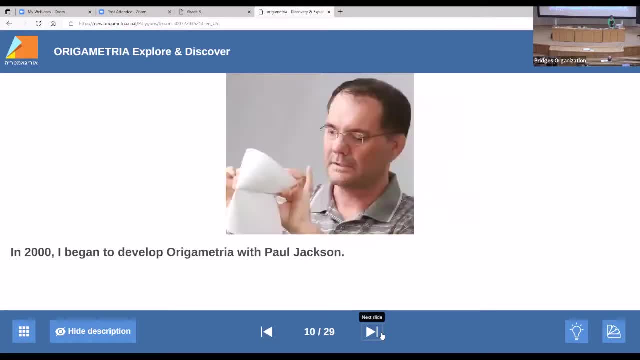 and i start to spread it around. and in 2000 i went to origami convention in germany and i met paul jackson and we got married. five months after he asked me to marry him by making a origami ring from half a dollar butterfly ring. 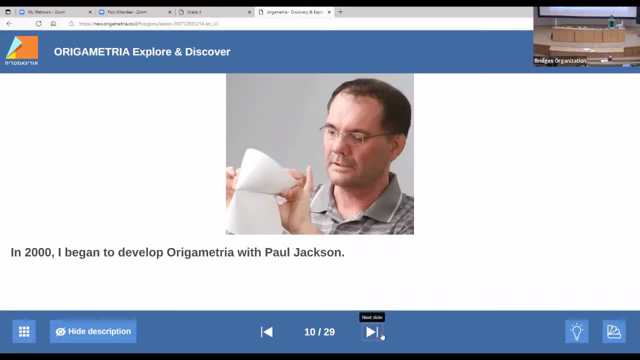 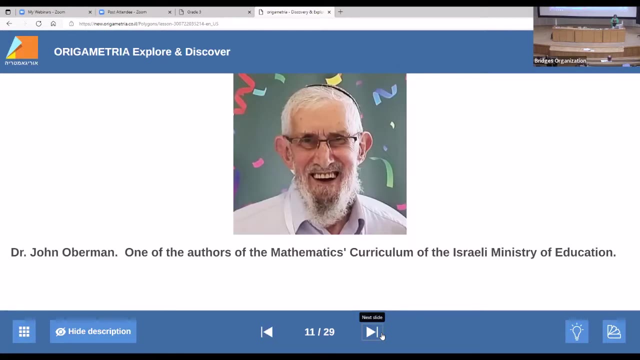 so we work together. he we have a two different area. you hear about him soon, but we also have uh working together and he do a lot of work for your material. this is dr johnny oberman. i feel a privilege that i'm working with him because he has 60 years. 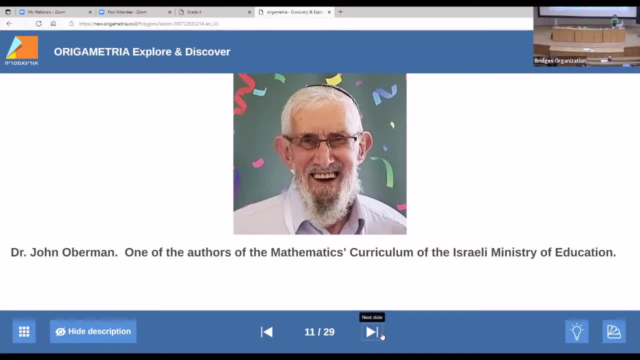 of an understanding and develop a curriculum in a maths education and he developed origami with me. we're working together and i feel i put in origami dr johnny oberman legacy of the geometry learning because he look on the geometry from the eyes of the students is very 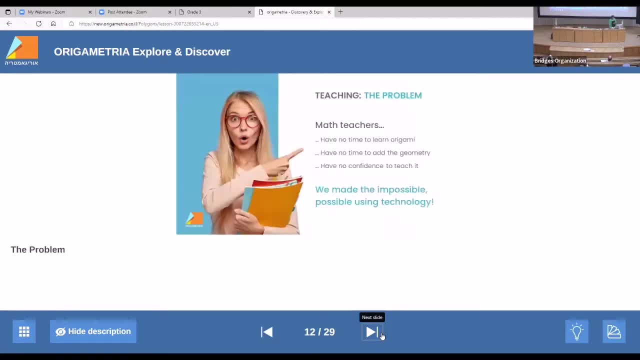 important and but many people who's doing origami say i try to convince the origami is good and they all the time get the comment nine. so it is a problem because the maths teacher very, very busy, they don't have time to start to study origami. they don't have confidence. 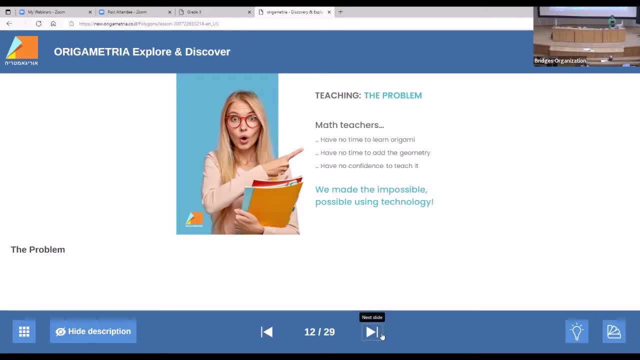 to teach origami, and yes, origami, it's a good tool to teach geometry. but how? yeah, so how we can make the maths teacher to teach. so in the beginning, i develop a program called origami to develop a learning skill. i teach in a special education school for 20 years and there's, i develop all. 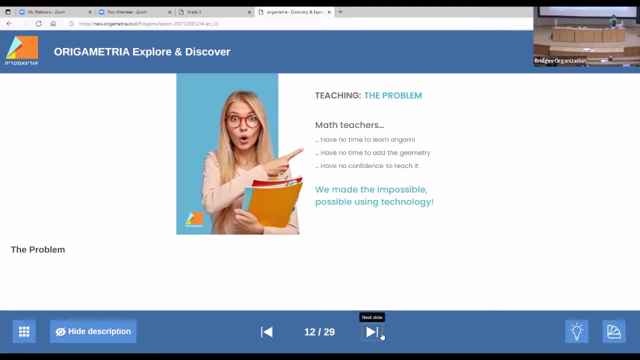 my teaching methods. they are very unique, so understand. the teacher doesn't have time for origami but, as i saw, i show you the lesson you understand she doesn't. if she wants, she can go into the lesson, put her on comment, but she doesn't have to, she just can come to the class. 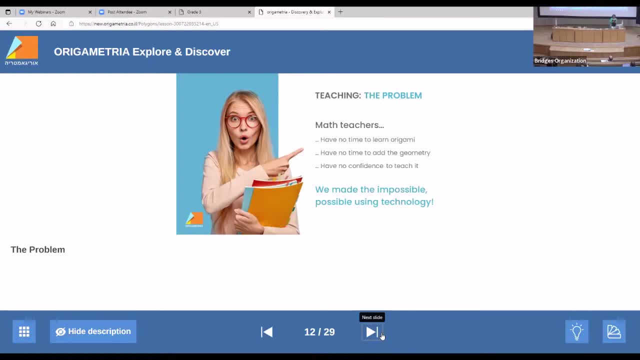 screen it and teach it and part of the problem that the teacher bring all this misconception to the children and when while she teach with that we make sure that she's accurate of the teaching and in maths is important. so um, also another problem with the origami teaching geometry is 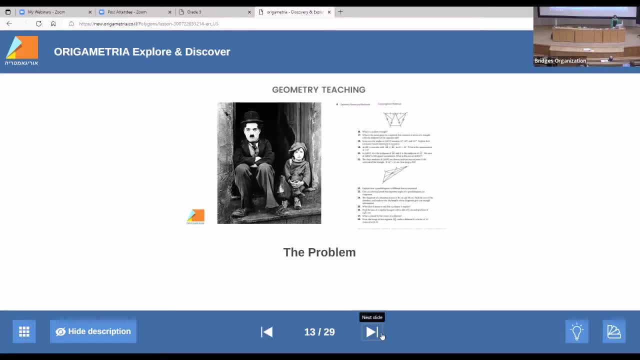 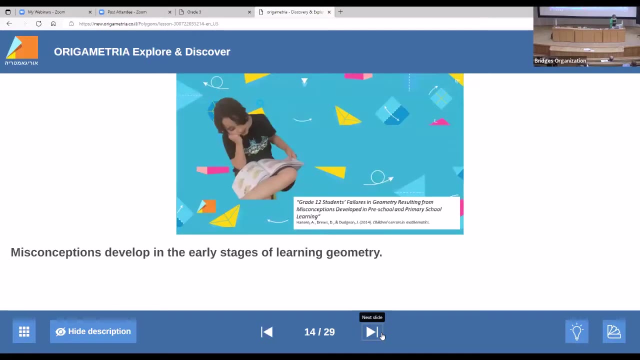 it's, it's even the try to put animation and something fun. it stay on the board. and also they still use books and the way they teach geometries makes geometry boring and geometry is excitement topics. so part of the problem the the misconception of the student. i'll give you example. um, before i show the example on the on the screen, i went once to 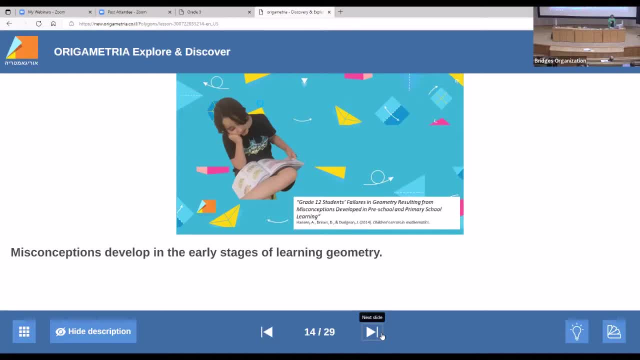 get j retiring one of the students. tell to the teacher: if you hold the triangle like that is a right angle triangle, but like that it's not. if you go to the class and you ask the student, what's that? the students say it's a square. what's that? it's not a square, it's a rhombus. 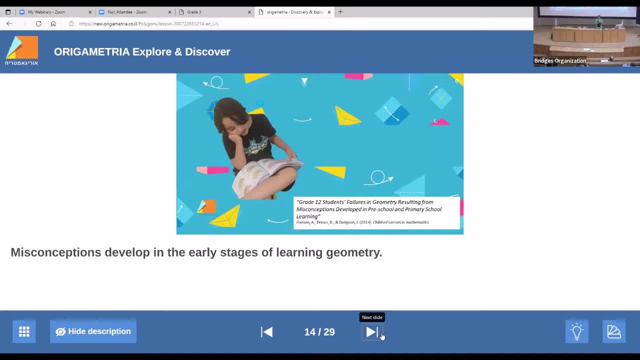 you know how i change it. it it's very nice. i said to them: okay, why is this? well, because i have an equal side for equal side. have right and again, and i check it with the measuring- okay, now we move it like that is anything of the square character, of the square change. let's try. does it still have equal side? 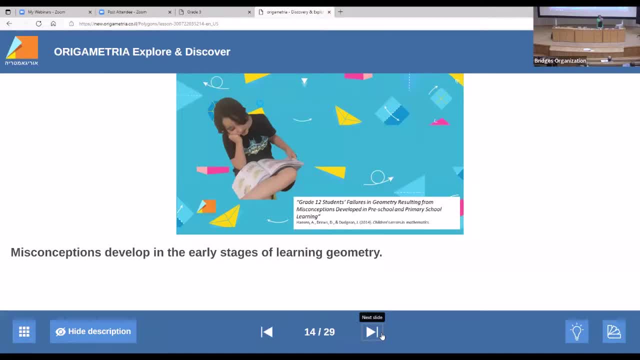 you still have the right angle. so my name is miri. when i sit, my name is miri. if i turn to the other side, i still say, really, and that's it, it's gone. they know and they understand. it's so the misconception, it's a big topic, it's part of the reason that the student fell in the exam. now you 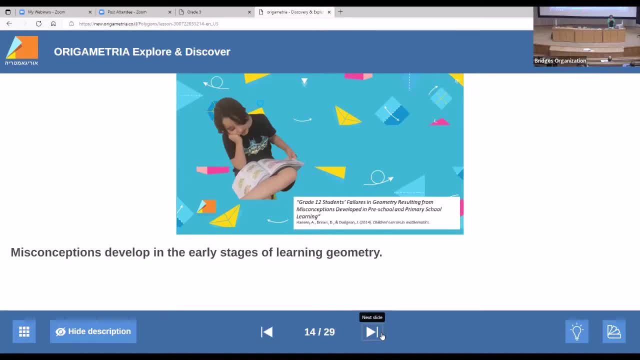 have to understand. many people- and i know there are many, many foundations- put a lot of money in middle and high school in to improve the geometry. but the problem is not there. the problem it's in the kindergarten. we need to start to teach geometry early age for able to start. when i was four- and i do believe- 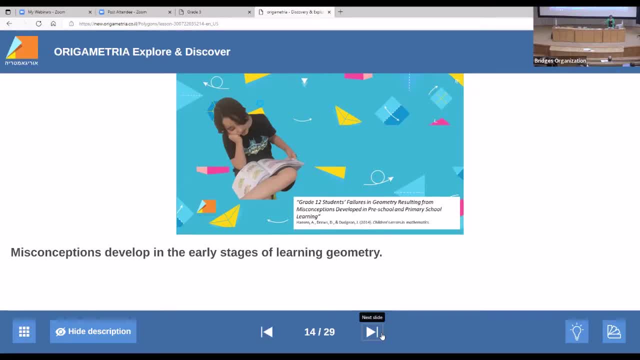 you need to start four years old to see geometry. if you teach good geometry in the early age, they have no problem with it. growth- because to understand geometry we need to understand geometry- also a good imagination. and and when you do it when you're young, then it's much easy for you. 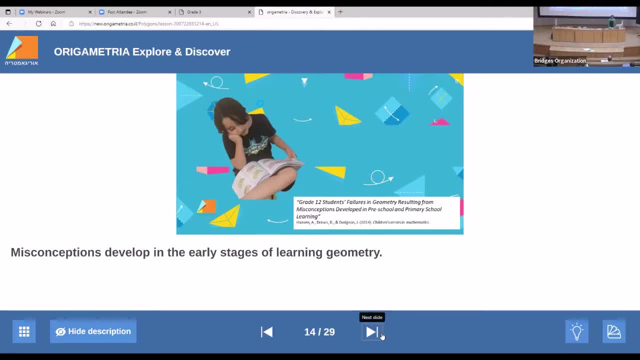 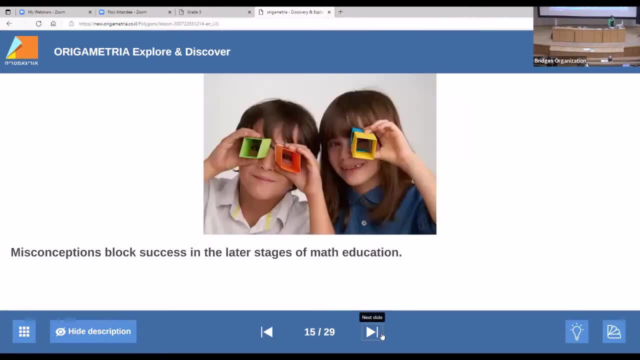 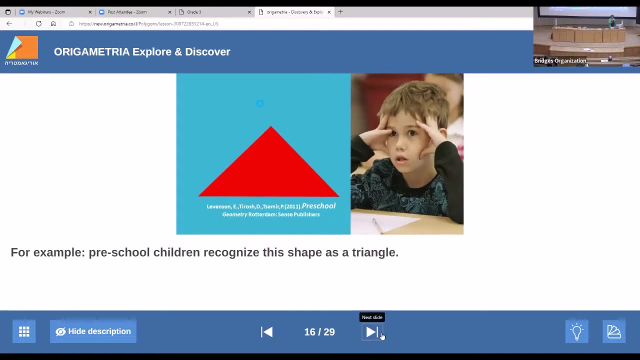 if you talk to kids four, five, six, they have really amazing imagination. it's helped to understand the geometry. so i give you example: um, this triangle. this is a research who have done tel aviv university, i think, um so they show this to the children kindergarten, if you have children about. 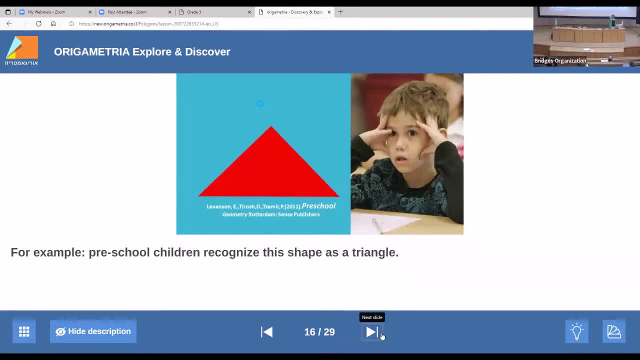 four, five, even six. ask them: what's that? they say it's a triangle. why? because always they show them a triangle like that. and now you ask them: is this a triangle? or even you show them like that, they say no, it's not. because all the time 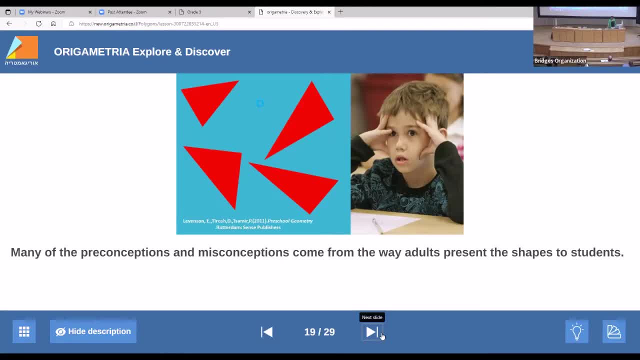 they show them the same shape of a triangle. it's all the time like that. so if it's all the time like that and you move it, they say it's not but how we teach them in. we say okay, we don't ask them if this is a triangle. we ask them: can you count how many? 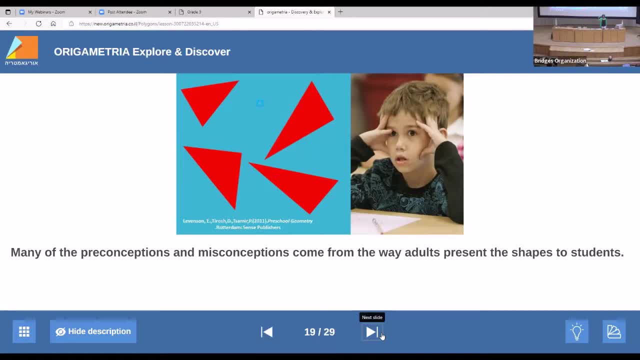 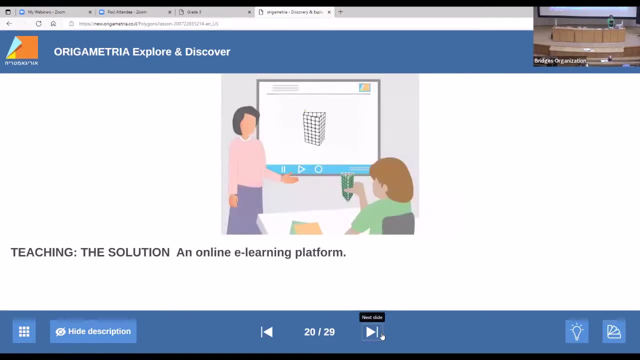 sides you have, how many vertices you have. then you know they understand the shape by investigate the same, but not by memory. so of course, the solution for all this misconception it's the origami online. it's easy to use, very friendly and also make sure the misconception doesn't go. 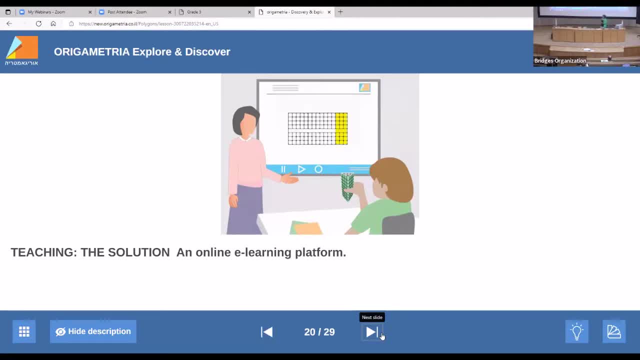 because we are the teacher who do it. um, i did with the dr john yoberman. i trained a lot of maths teacher and we asked them: how, what is the definition of an angle, how you do it, what is the definition and the way they explained it. you see in the in the pizza exam, the result: yeah, they say it's a corner, two line come out. 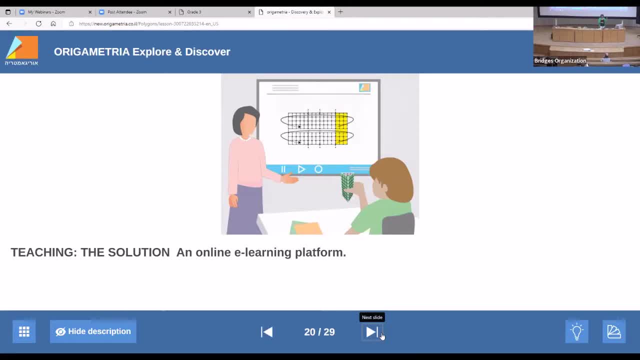 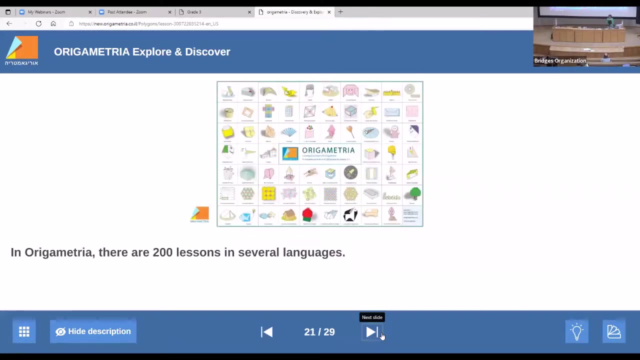 from the corner. okay, so the children say the length of the angle is the angle or maybe the distance, but the angle is the distance between one to another. so when we do it with our origametry it's much easier to escape all this misconception. so we have over 200 lessons each model here. 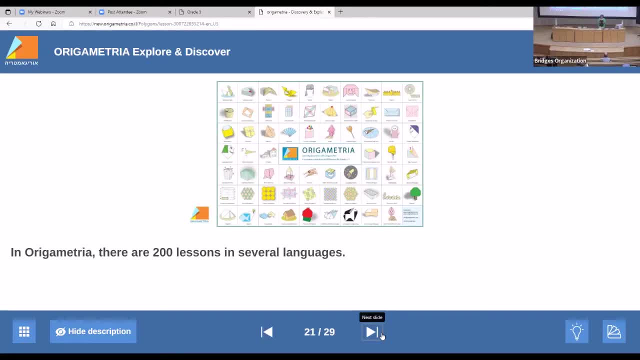 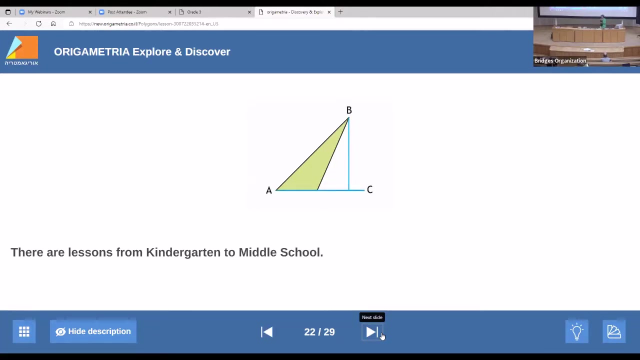 teach some topics and it's attached to the curriculum in maths and actually all the curriculum in education all over the world is the same. i've been teaching in many, many countries and i know it's the same so so we have 200 lessons in each one teach different topics from kindergarten to 7th grade. 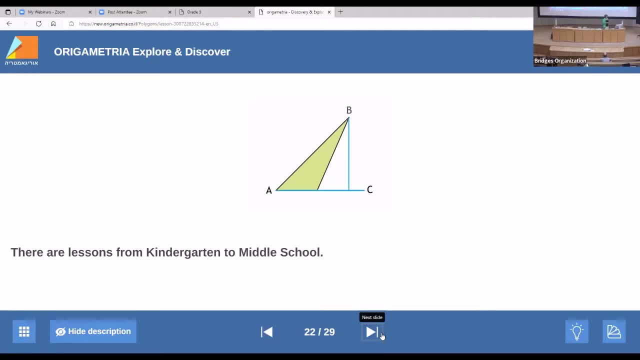 like this one. they make a finger um nail and they learned about the height of a triangle, or here to do tiling. it's a fifth grade usually. so the that make this tiling beautiful less than this one or this kind of tiling. so i've been asked by one of the 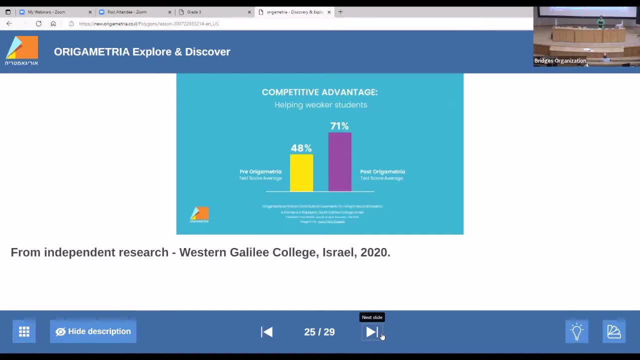 professor to go to school and teach there with her. in the beginning she was very negative: what i'm doing with this origami, i'm a math person and all this. so we did teach and she saw what happened to the student. she saw the knowledge. then she did the research about origametry. 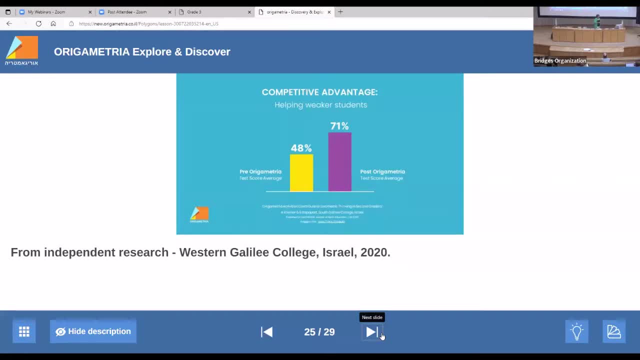 and she wrote a few articles about origametry. so what she did? she just did it before covid. she took the weak group and strong group. the control group was a strong group, it was about 71 percent and the weak group was about 48 percent. she used few population: arabs and jewish. 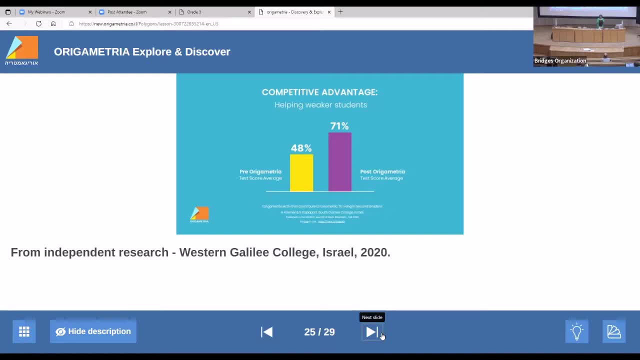 and she saw after a very short time the weak group have the same result as a strong group by study with origametry. so it's reduced the gap between the strong and the weak and we know after covid this is a very strong topic because the strong people can manage, can take private teacher. 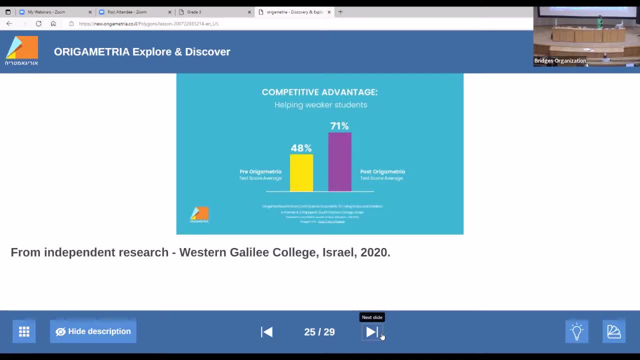 can, can, but a week don't. so i know this year is going to be another few research about origameteria i've been asking. of course i have nothing to do with this research. they do independently and even the college buy the membership for the origameteria and do the research. 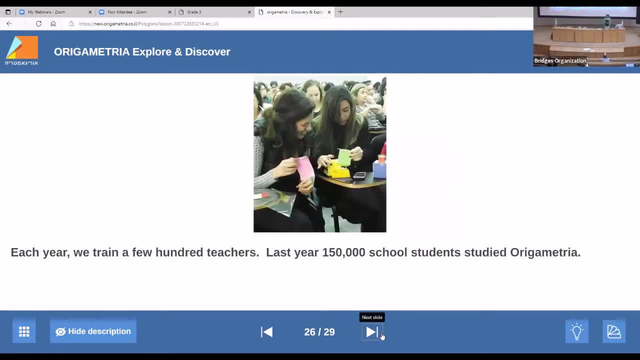 every year i trained um hundreds of maths teacher. it's nice than last year. i don't need to drive anywhere, i just do it by zoom. before i used to take the train few hours to here to here and it was all the time on the road, but now i do everything by zoom. it's nice, so we train a lot. 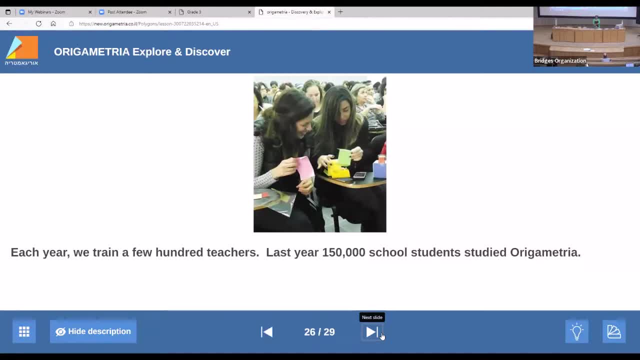 of maths teacher. um, we don't train them because to to use origameteria e-learning site is very easy. it's enough one meeting and they know how to use it. but also we work with them about the geometry learning and all this, and i do it with education ministry courses for teacher. so we train. 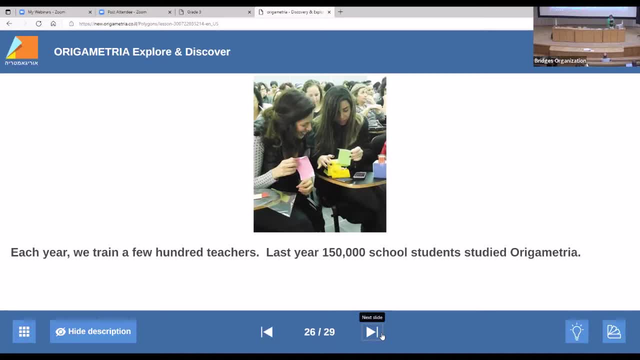 every hundred of teacher. we have 150 000 students of study geometry with origami every week. it's amazing. huh, it's nice. yeah, i'm very proud of that. you can't believe i woke up in the morning and that's what i do, all right. 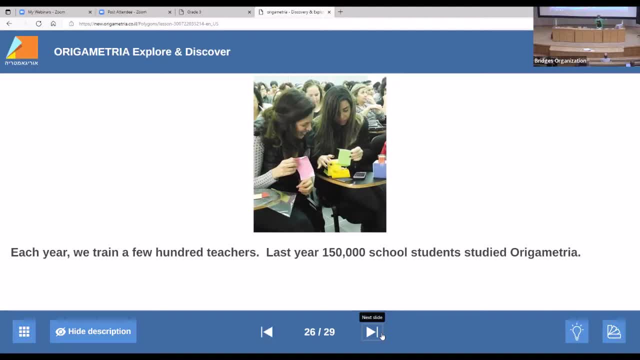 all right, lesson with dr johnny oberman, develop with paul the models, and i just leave that and i put all the lesson and work in it. i just eat and live and breathe this. i look at the, i look at origami as a work of my life. come on, bring me my best husband. you know i want, but but origami it's. 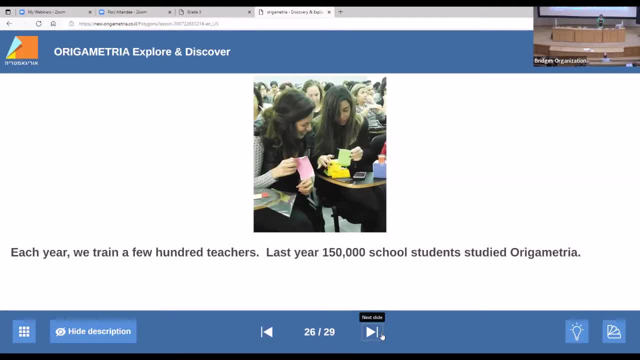 amazing. amazing too, but if we use it not from the origami side, from the education, because sometimes origami people come with the excitement and they need how to excitement and teach it. and i came from the point of the education ministry needs what the student needs, what the system need to make the 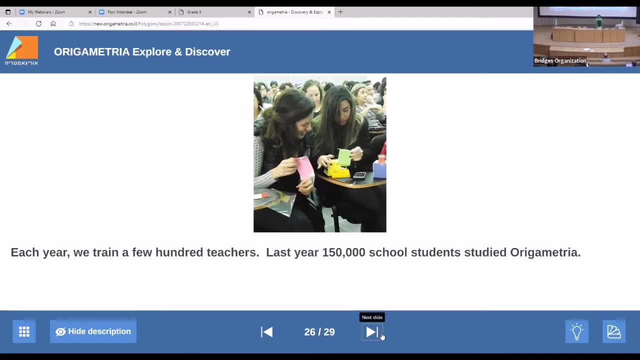 student, better learning and joy. because in the beginning, when i came to the education ministry and i said, look the children happy when they're studying, i said: look the children happy when they're happy. it's smart. they need to learn what's happy. um, so the joy is very, very important. i'm not talking about the motor skill. 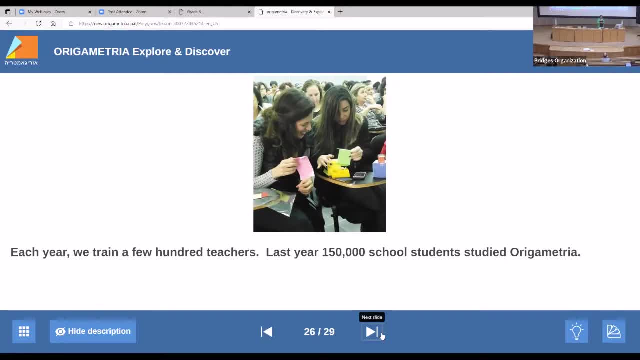 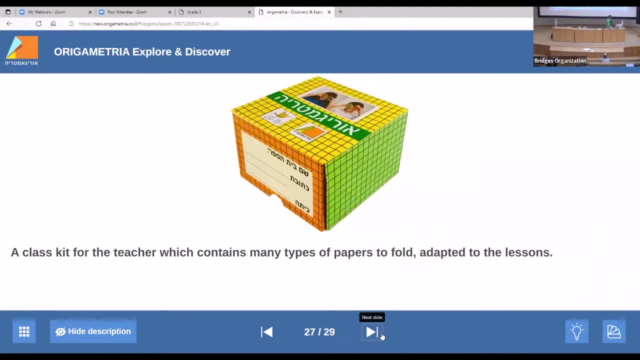 uh, space awareness and all the other learning skills that when i was starting with origami, i was really emphasized that i don't emphasize them because it's in plant in origameteria. so what you see here, you got paper for me. yeah, the paper you get, we print them in israel. i refuse to buy paper from china or from. 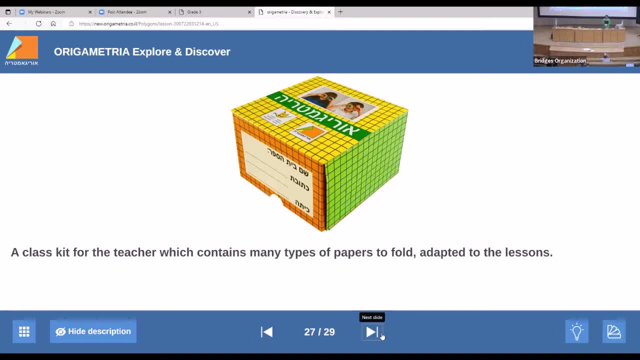 other places. we print them in israel and the people who pack the paper. it's a handicap and it's very important to me because it gives them work. many times i go to the place they are packing our paper and i'm very happy that origami is a way to protect and cook our children and our 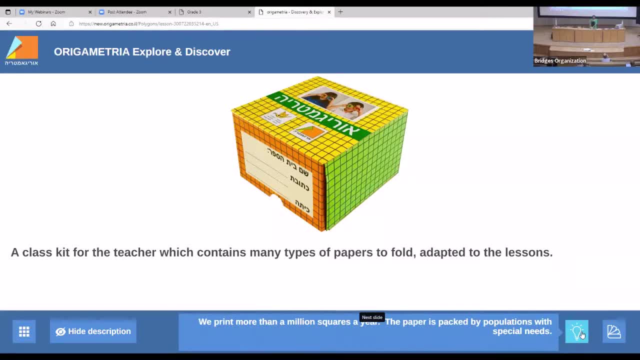 children and all our children are different and i am very happy that origami and the people of origami of we built and finished the origami society and i am very happy that origami based on origami. it was helping gosh. They wake up in the morning and they have something to do like packing our paper. 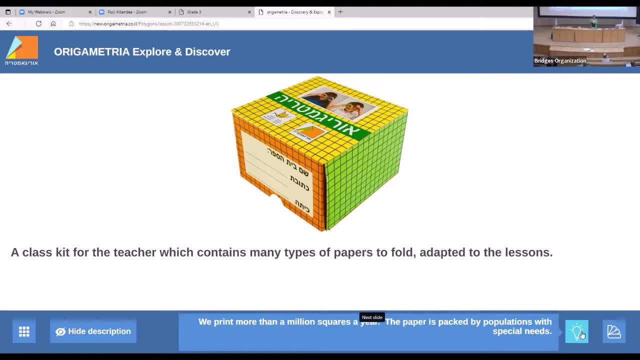 So every teacher of every school who buy it, who buy pack like that with this paper, Some of the paper it's a paper like: if I want to teach just a minute, if I want to teach the children measuring, 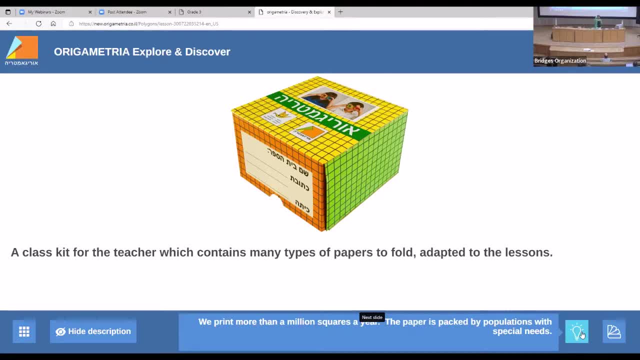 So we have a special paper that each square it's one centimeter. so they can learn that. But you know this: if I take two paper, put it on each other, they're equal. And now I fold to a triangle and I fold this one to rectangle. 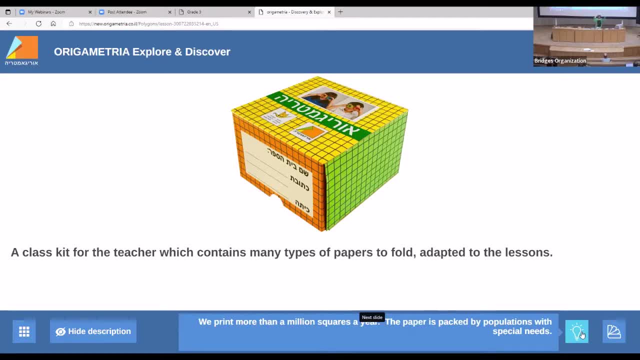 And I ask them: is this area equal to this area? No, they're a different shape. Yeah, But when they see They are the same, I rotate them and you can see: And this is a half of the same square and this is a half of the same square. 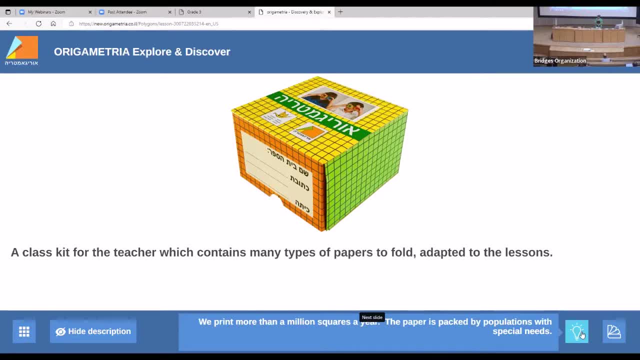 Then we know they are equal, even it's two shape. So we have a lot of lesson with the square paper that we do three different size but they are equal area And then the children understand it. We also have special paper with a dog. 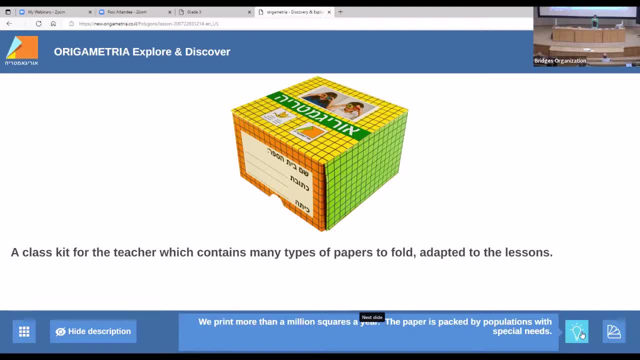 So they can build and work out how to measure with that. So this part come and it's suit to each class. It's a lesson. It's according to the lesson, Of course, origametry. I want to go worldwide. 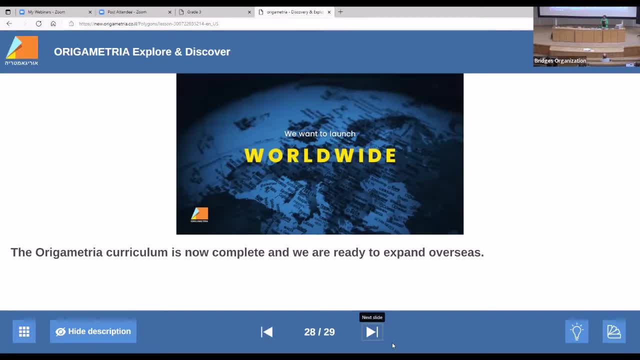 So any one of you, if you're in your country, you know people you think origametry I can feel. Please, let us know, because in a new digital origametry e-learning site we can have any language easily, very easy to turn it to any language. 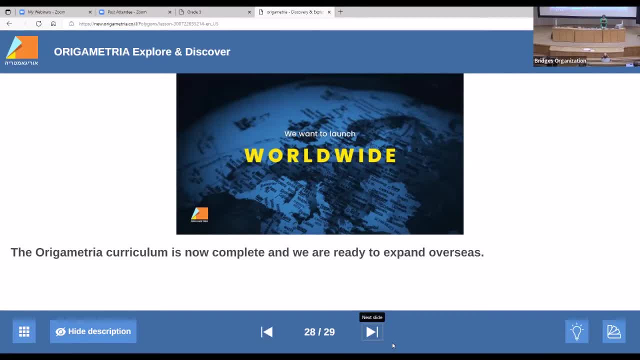 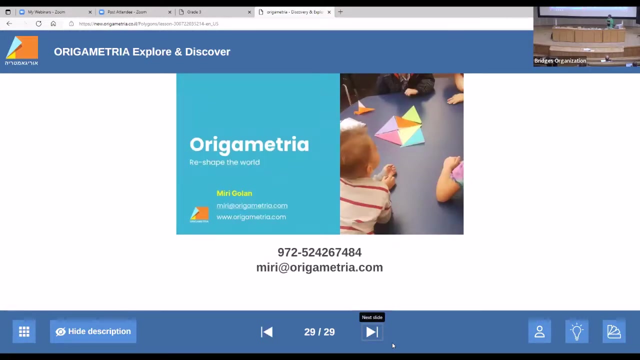 And we do believe that if children learning by playing, investigate by doing like that and the teacher teach like that, it's be better result in geometry And geometry is important topics. So if any one of you want to have a contact with me, please do. 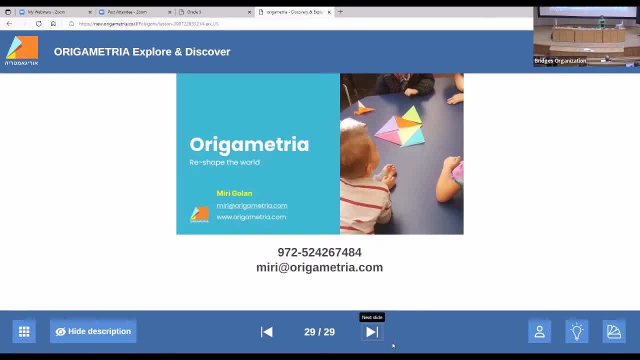 And you got here the Jackson cube So you can take it apart and build it if you want. This is how we give away to the school to show them: Yeah, it's origami, It's fun, But this origami It's fun. 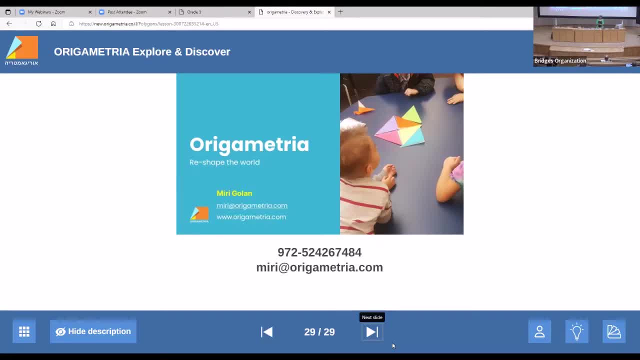 But this origami, It's origami. teach you geometry, So I hope I open you some window to origametry And thank you. If you have a question, I'm here to answer. Thank you for that great talk, So we'll start here with Eve. 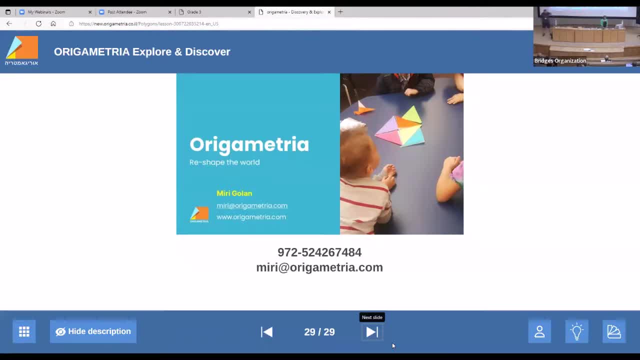 No, they need to repeat the question. So the question was on the cost of the curriculum, I think if anybody want to talk to me. but yes, it's cost. you know, all this cost fortune to make the animation and hours of work. 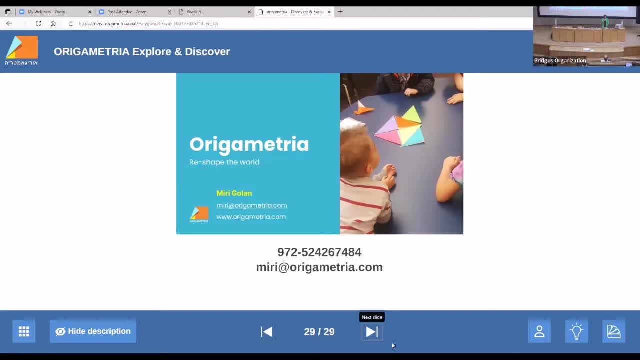 So yes, usually school buy a membership for one year. Say: any job doesn't necessarily help you pay for the course. I'm so sorry I missed all the questions that weren't even mentioned. Can I talk to you later By? somebody wants price. talk to me about it later. 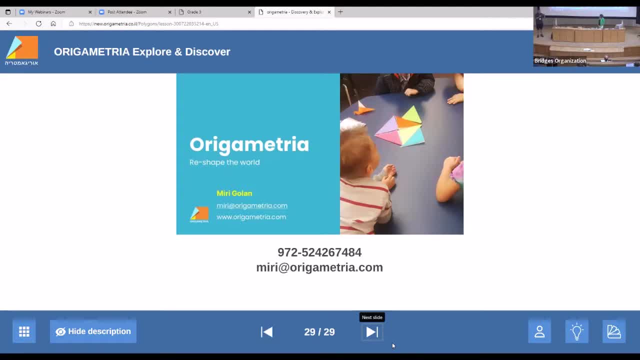 It's not. Yeah, So the question is about other topics beyond Origami, other topics beyond strictly geometry. Yeah, we started talking about. Okay, That's fine. Okay, Go ahead to make a session. um with fraction, prepare the student for fraction, the problem with fraction. 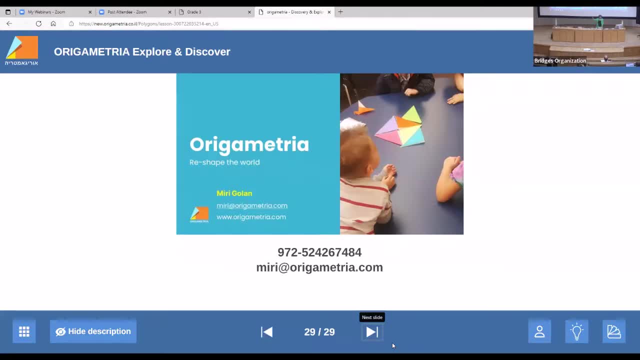 that the teacher run to do quiz with the student before they understand what is a half, what is three quarter, what is so what we did? we build a session. who build the geometry, understanding of fraction? so they can do. we in the middle school we did go up and i think this year we're going to. 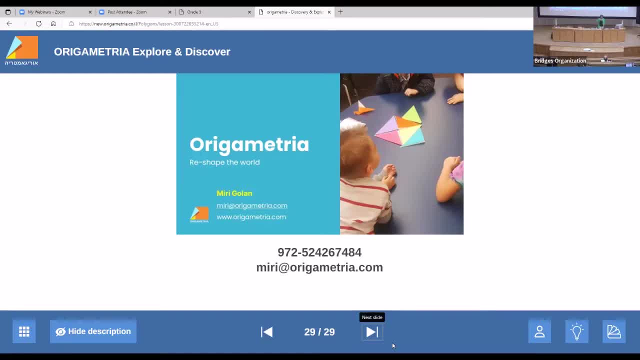 go and fill up more lesson to middle school and up something every time. we give more and more to higher mathematics, and also not just geometry. touching the mathematics. paul, you have question. so the question is about, uh, how Orgometria helps children with learning disabilities. I start my way in the special education school. 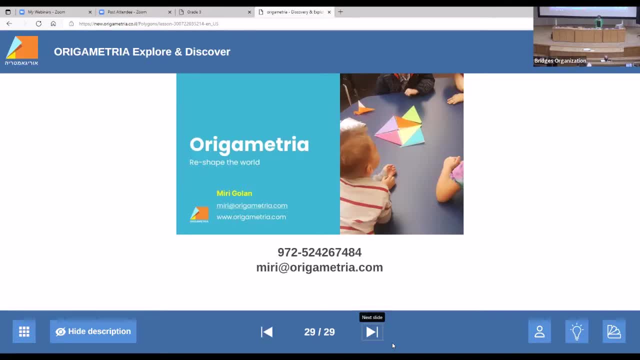 Children was there from intelligent average and up. but emotional problem and learning problem. Orgometria is very, very good for students who have dyslexic learning problem, hyperactive emotional problem. We have a phrase that I really like, So when I start, I start origami, also as a therapy. 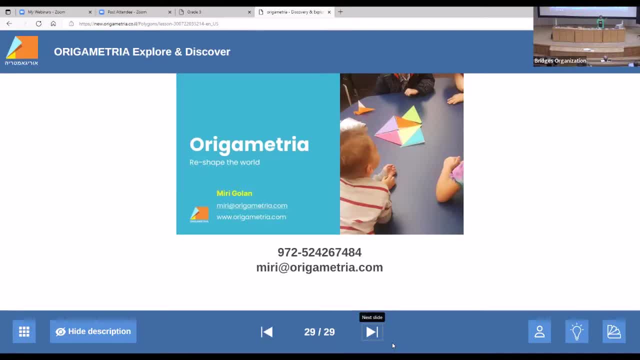 Yeah, And many of the students I teach. now they are 30 years old And it's amazing what they tell me. this changed their life because they start the learning with Orgometria with me And then they saw they can succeed and go to the other area. 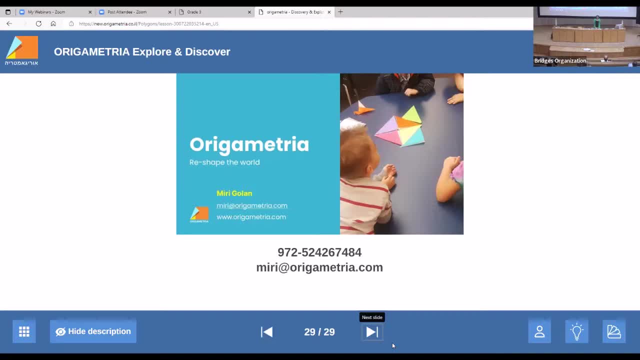 So the phrase is: when the paper fold, the emotional unfold And it's everything you know. So in special education, yes, You can use it, And we all the time hear from the teacher- I always have kids in the class who doesn't work. 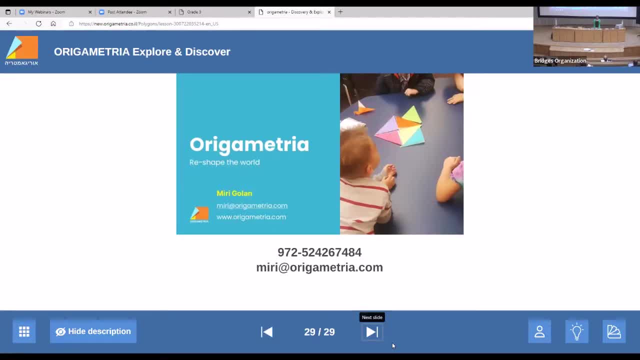 He's not good, He's make a mess, And when Orgometria start, he sit the first and he have better result. So it is very good tools. Yes, Yes, Can you ask a question? Yeah, Yes, Way in the back up here. 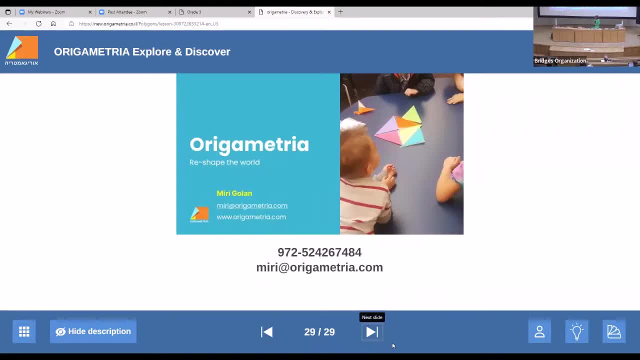 So the question is: are there learning theories that are used to frame the student thinking? Yes, I have a question. Is there a question back here Or did you have a question? Yes, I have a question. I had a question. 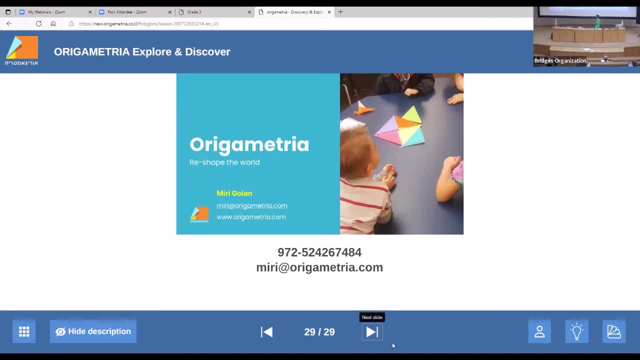 Did you have a question? Yes, uh, ah, okay, yeah, we, we do teach, uh like vanhila. you know when, when the children um start to, when i train teacher, i talk about vanhila a lot because i think it's very important they did it. 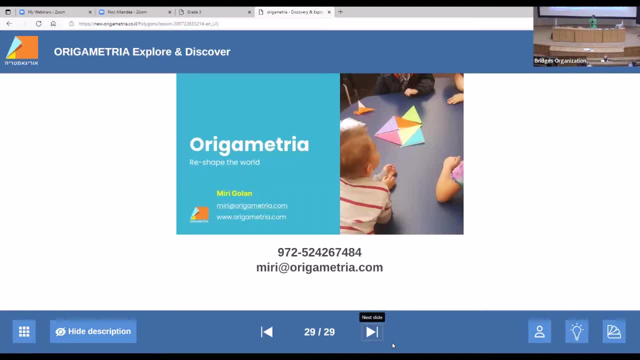 in 1950, but still relevant, yeah. so sometimes the teacher uh escape, uh don't teach in kindergarten, don't teach first and second grade start third grade. now they need to understand angle, but they don't know what is a polygon, they don't know what's the size, they don't know. so a lot of 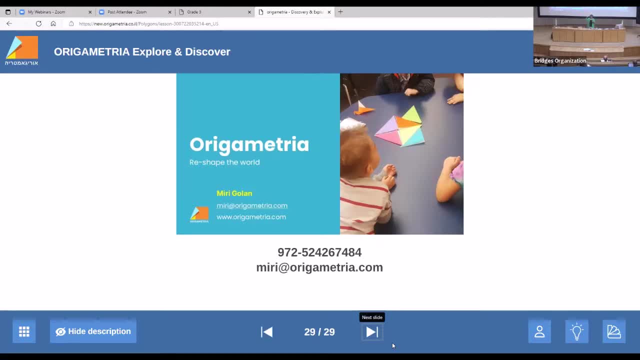 material is missing and while the teacher teach and the children doesn't understand, it's not because the children have no ability, it's something missing. i always say to teacher when i train them: when you try to teach something and the student don't understand, don't continue to try to explain in the same from a different direction. check what he missed. 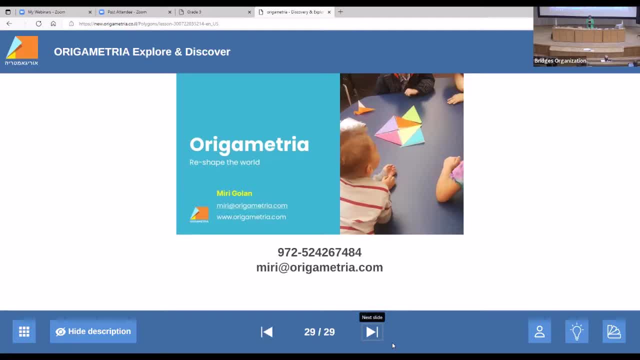 what's missing of his understanding. now i asked the the: if you, if you understand what's missing and you teach him what the missing material, he'd be okay. and i asked my teacher: what's the most important thing happen in your class? there's so many things. 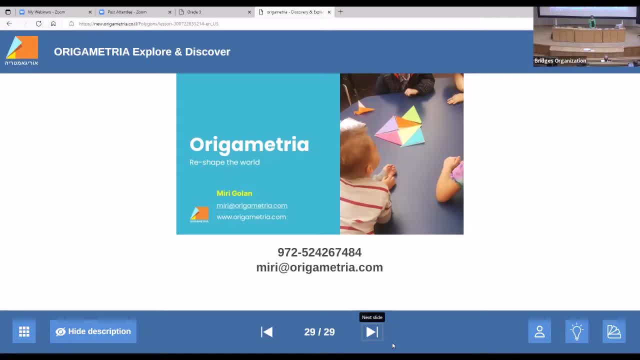 except one. it's the student answer. if he answer me and i listen to his answer, i know what he doesn't know. i know what he know. the answer is very important. you know the education system run too much to exam. they say exam 60, 90, 100. what it's mean, what it's about me if i have 90 or 60? 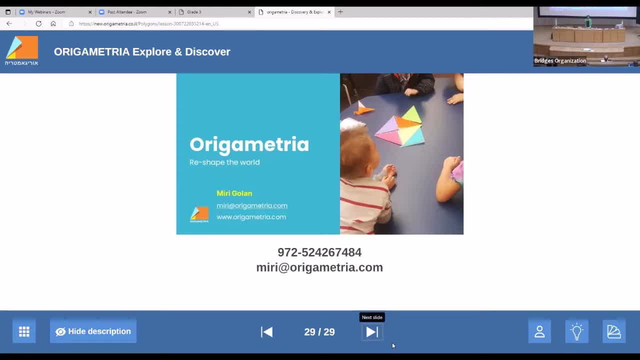 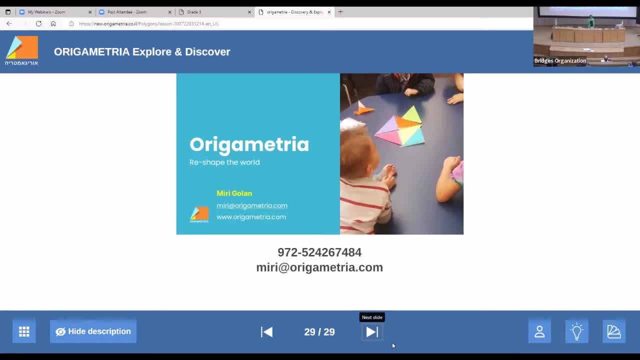 that is, the student is good or not good, and this is wrong. that's why, when my son came up to me within 160- 40, i never say to him very good. i always ask him: are you happy with that? this is what you want, is it okay for you? and sometime he got 70 and he said: 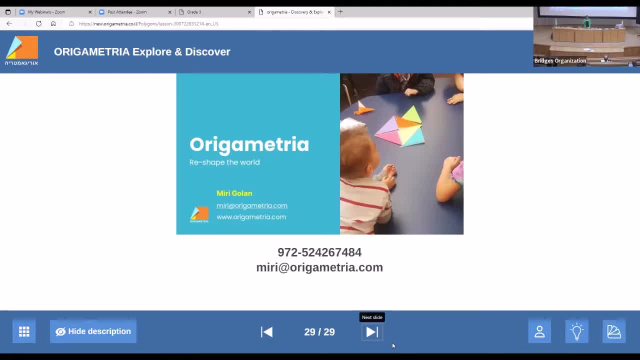 i'm very happy and i need to say, okay, it's very important not to so all what you talk about um, vanilla and teaching um according to ability of the student. it's very, very important to understand that, because i see many teachers who doesn't understand it. 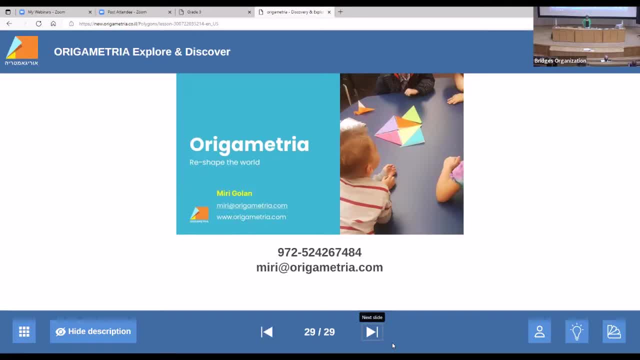 they try to explain that the student doesn't stand, say, oh, he's not good in math. it's not true. everybody can be good in math, everybody can be good in geometry. just teach right, yeah. and i think the question is: is this, uh, this teaching methodology, uh helpful in students? 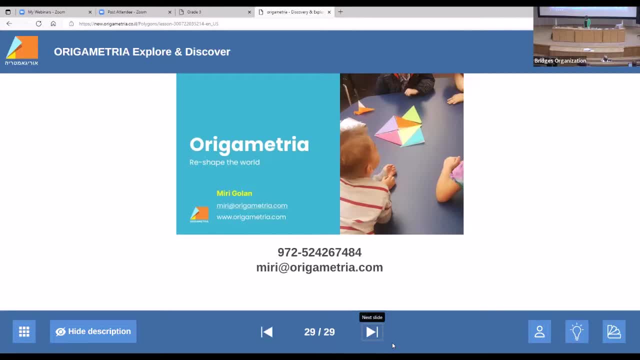 constructing proofs later on in a more formal way. oh people, i just had a question. so are the, when students are doing this, um, do you have evidence that perhaps later on during their decisions and sig slipping data is going at, perhaps later on in school, that they do really well in terms of being able to formally prove? 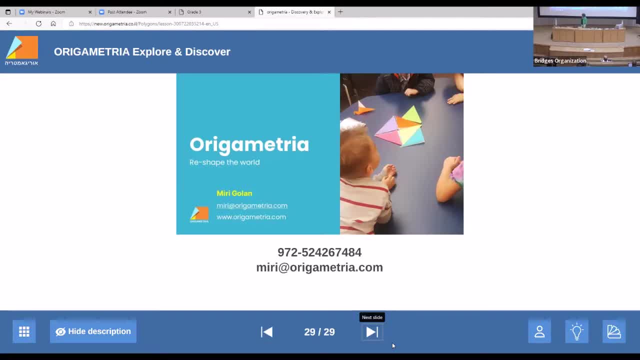 things in a written way in a geometry class or subsequent courses that they take. The thing is, before they did the research. I knew it. I heard it from the teacher, Because if the teacher buy it for the four years, it means you're doing something. So we hear that. 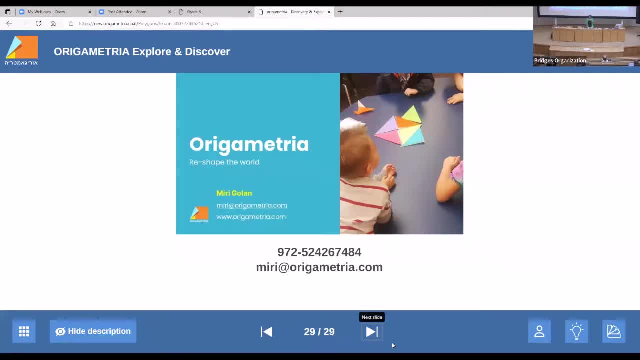 all the time. I'm working with that for teaching with origami for more than 30 years. I see all the time that I hear my students when I was young and I was teaching them. So yes, we know it, but it's. 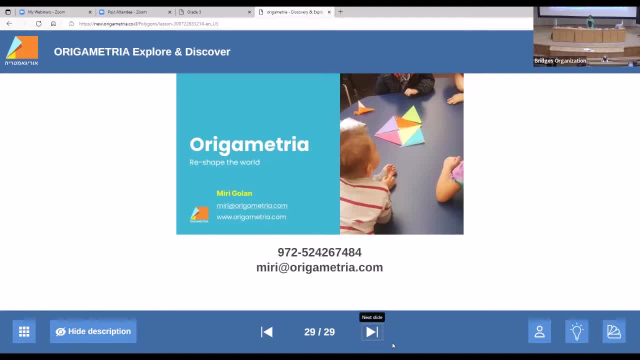 not enough that I tell you that I improve and they come to me. The most important is be more and more research about it. Then people believe it better. But yes, if you use it and you know it. you know what I said to a principal, because sometimes teachers have to say I don't want to. 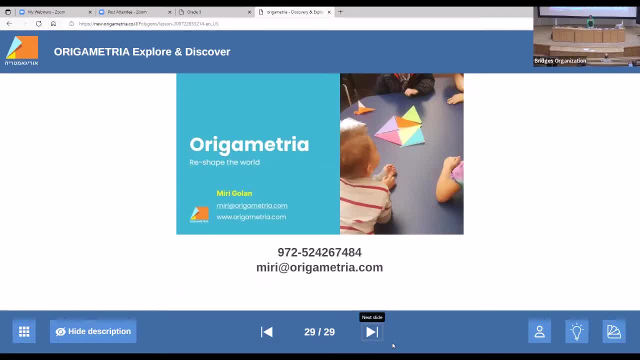 teach it. I don't know if I succeed with origami and all this. So I said to the principal who buy the program: tell your teacher that you're going to come in the lesson that teach origametry, So they should teach and you come. You don't have to come, It's enough. you tell them, you come, or. 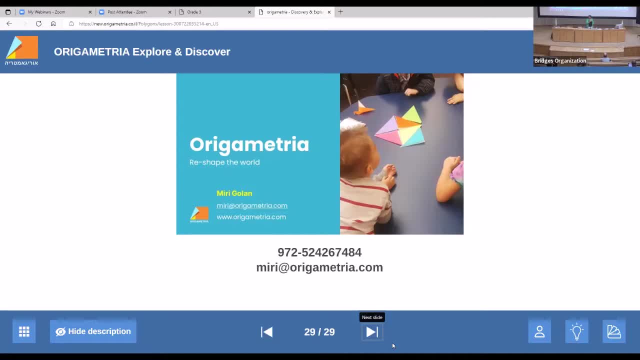 maybe come for five minutes. So if the teacher know the principal come to watch her, she start to practice And start to teach What's happened. when she start to teach The children get crazy about it. They don't think they enjoy the investigation of the geometry. They have some origami model. They 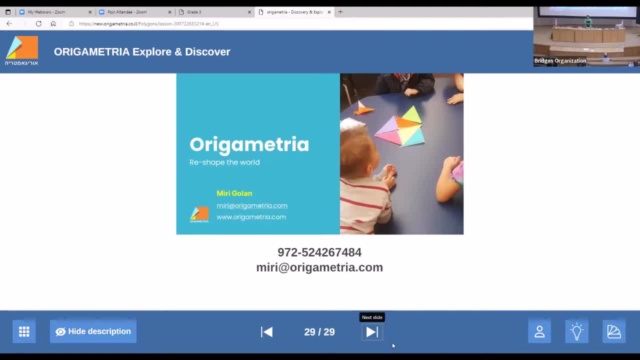 love it And then start to knock the teacher. Can we study origametry? Can we study origametry So it's came from the children and put pressure to the teacher to change, to take something she doesn't know, that this can improve. 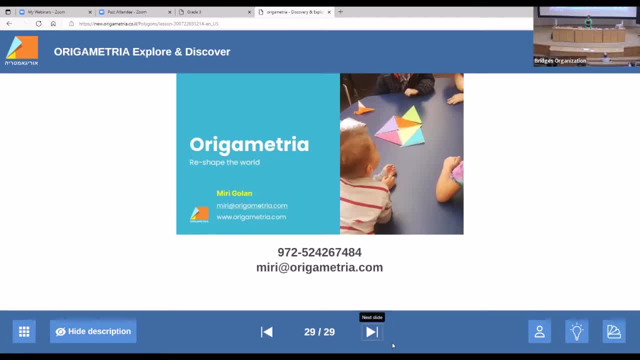 And after she give them exam and she or the math supervisor in school suddenly see the result is up, Of course they take it. So the question is: what is the debugging process for the pedagogy that is involved in the orgametry at the org? 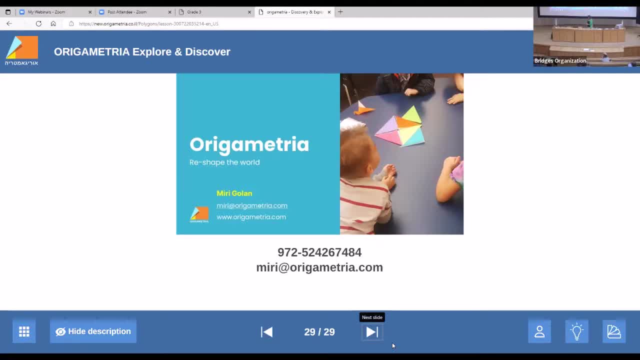 Orgometry, or you give example that the chemical was used in the first time. So you, you change the process. So yeah, there's a example that the students fall wrong on what you do. you know that's what you mean, okay, um, after. 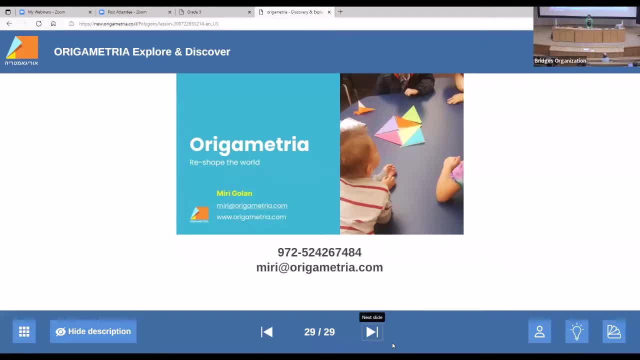 every step we teach i recommend the teacher to go between the student. we never say to them: it's beautiful, it's good. we say to them: ichiban- in japanese each is one, band is thousand, you are champion. now, ichiban is a word nobody use, only the origami teacher. she go between them. 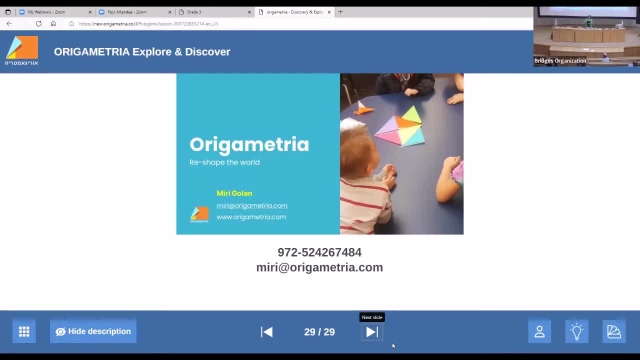 and in every step almost, and see she always go in a random way. she doesn't go straight to the kids. who doesn't succeed, because he feel like she helped me, she didn't help anybody. then it's become worse. so she make kind of a right all the time going in the same direction and she give 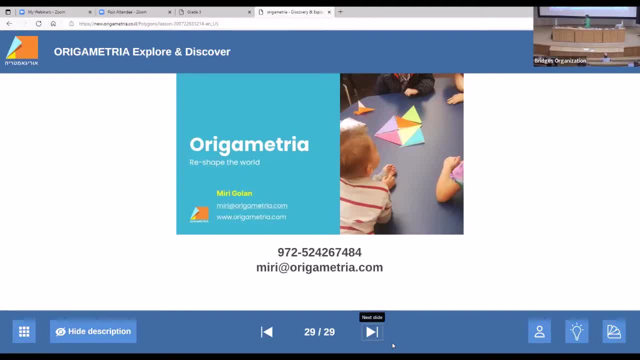 ichiban to everybody. so if i give ichiban ichiban and then he have a problem, if i stop a minute and show him with my paper, nobody feel and he feel more confident. so it doesn't happen that after few step that you find out that he didn't fold it right. yeah, we don't come to this uh position. 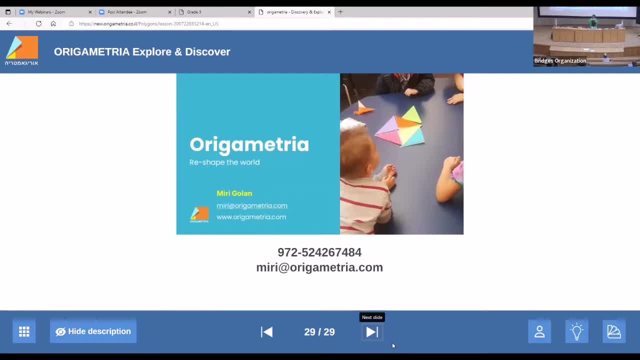 because we all the time see the student and go over: um, i hate the word succeed. very good, you succeed. i hate this word because when i work in a special education i ask the student why you didn't succeed, the answer i got: i'm not good enough, i have no ability, i'm not good. so when you say succeed or 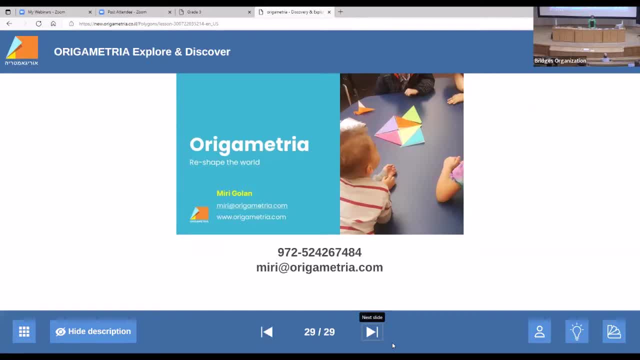 even you praise as you did successful way. you know i hate this word because the students stop to try, because what is learning to try again and again? and there is a word that i say it's old world: we learn from mistake. it doesn't work for the student what we learn from mistake. if i did, 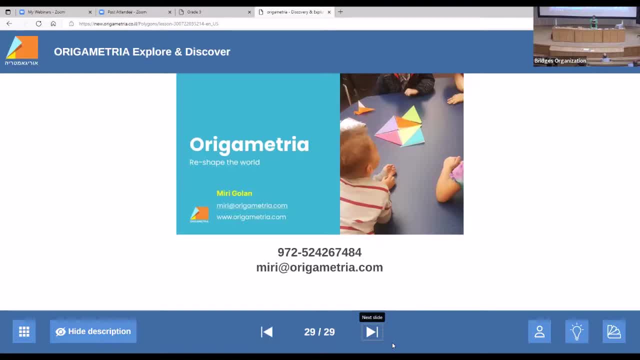 bad, i'm not good, and they stop trying. so i tell my teacher: open the window, throw the word, succeed out of the class and say: did you find it is discovered it? in hebrew we say it's a nice word. did you discover that? did you find it? 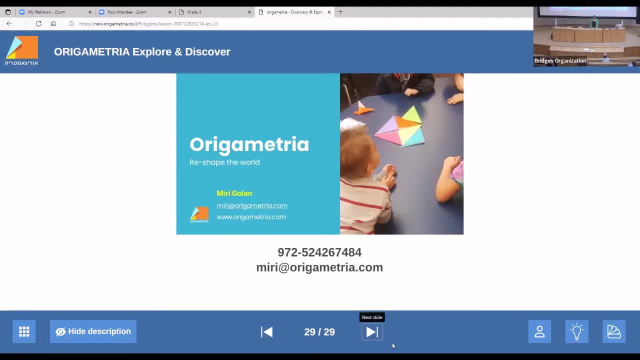 why so? ask the student why you didn't find it. i don't know. i find it later. why i didn't discover. i will try to discover after. it's not me the word success, it's my ability and i don't like it. so we take this word out of the class. i sometimes, i give you know, i teach the teacher to teach. 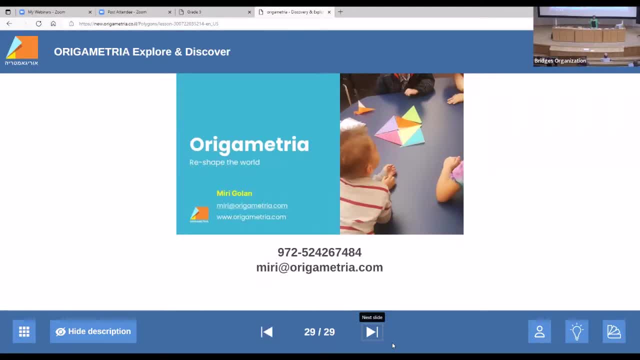 origametry. but many times i give the method. the principal come to me and say: you know all the things that i'm going to talk about it because i work 20 years in a special education. i have big understanding what stopped the student to try? we need the student to try all the time because